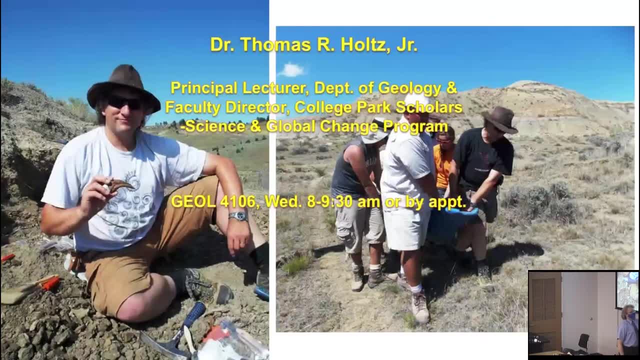 Pandemic brain. it's got us all. So who am I? Hi, I'm Dr Tom Holtz. I am a principal lecturer in the Department of Geology. a principal lecturer. He's a faculty member who is primarily employed as an undergraduate educator. 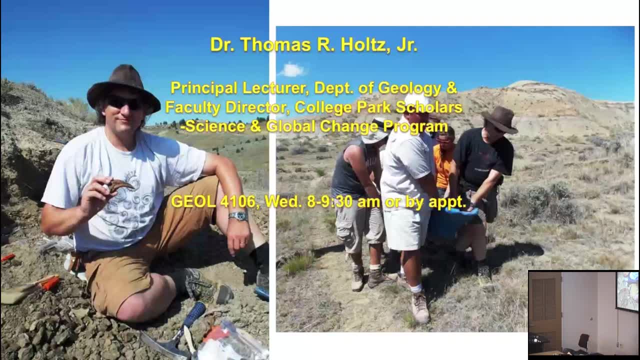 And I'm in the Department of Geology, which actually the Department of Geology is right over there. So if for some reason you happen to see me in my office, it's the next building over, right over there. I'm also a faculty director of one of the College Park Scholars programs. 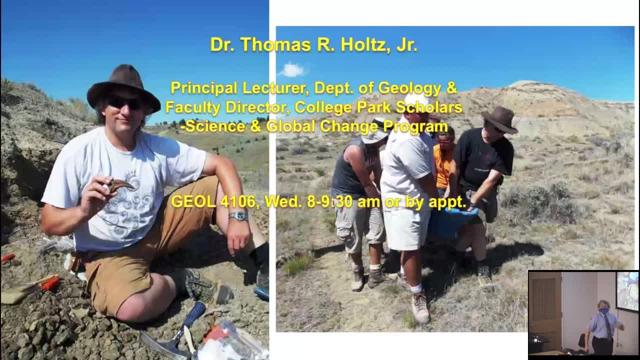 And so I've got an office over in Centerville Hall And it's one where you would need to be a scholar to have swipe card access to that, because it's actually a dorm. I'm just in the first level, So my office hours that I intend to do this semester are Wednesday mornings over in my geology office or by appointment. 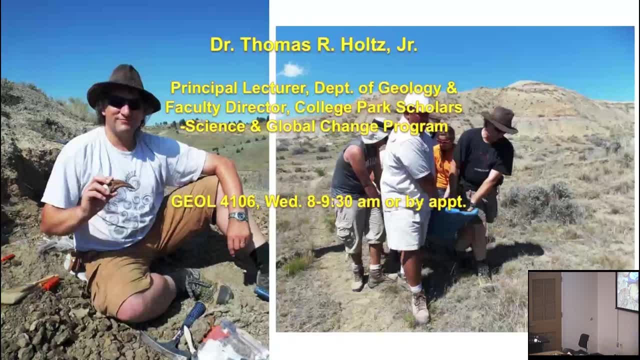 This would be my live in-person office hours, but you know, if you want to meet by Zoom at some point, it's a brand new world. we've all learned how to use it and it has its benefits. So actually let's back up here. 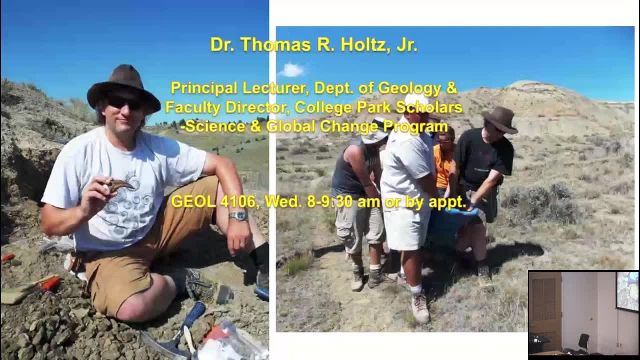 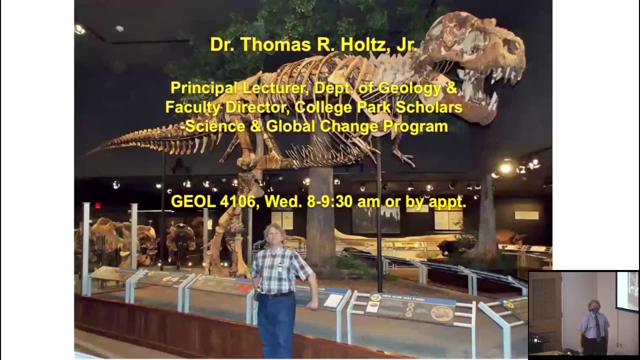 So I am indeed a paleontologist. I actually do this stuff for a living. So this is me out in the field in southeastern Montana with the claw of a very bird-like member of the meat-eating dinosaur group. My particular area of expertise are tyrannosaurs, so T rex and company, although I study all kinds of dinosaurs. 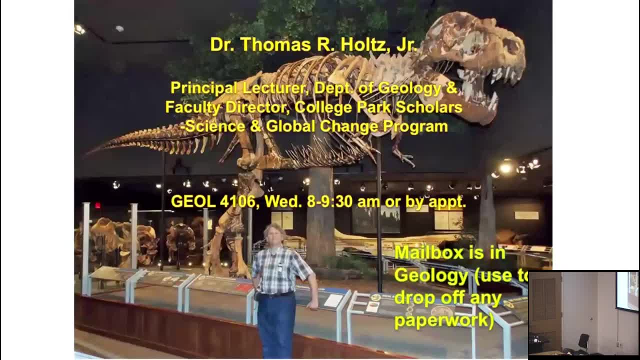 If, for some reason, you had to drop off paperwork, Remember paperwork, You had to drop off paperwork. My mailbox is in the first floor of geology, open during business hours. But yeah, I'm trying to make this as paper-free as possible this year. 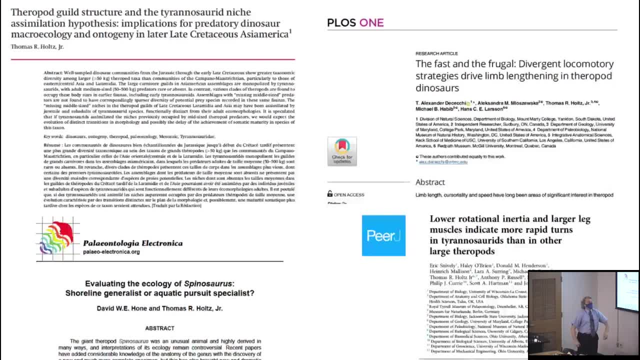 So, as I said, I am actually a researcher. I do study and publish on dinosaurs. So here's what four different papers that I was author or co-author on in the last three years or so, And actually here's some cool art associated with each of those papers. 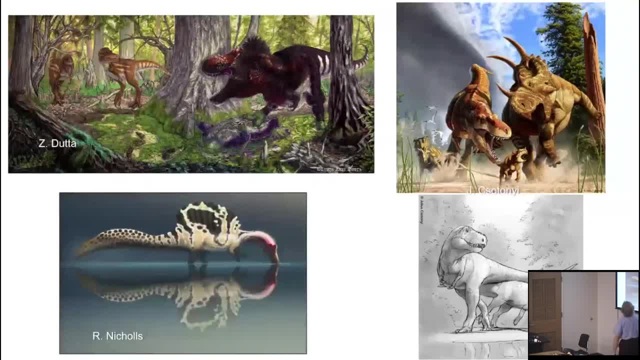 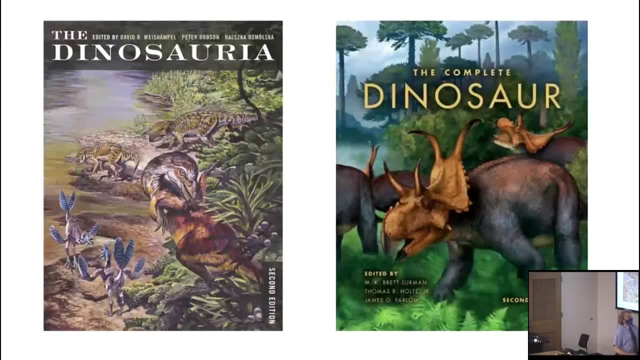 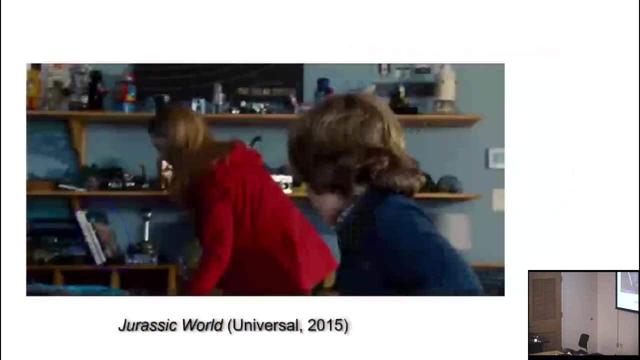 By various paleo art colleagues out there And you know I've published and edit in various technical volumes and also general audience volumes And one of my books actually has been seen by hundreds of millions of people, At least very, very, very, very, very, very briefly. 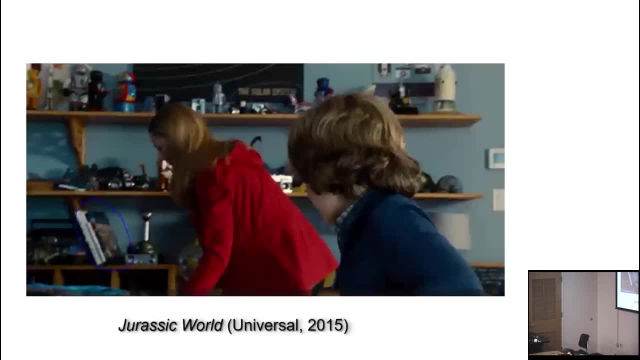 Because in one of the opening scenes of Jurassic World- you know the reboot of Jurassic Park- my book is right there in the background. If you blink, you will miss it, If it weren't for the fact that when I saw it in the theater, 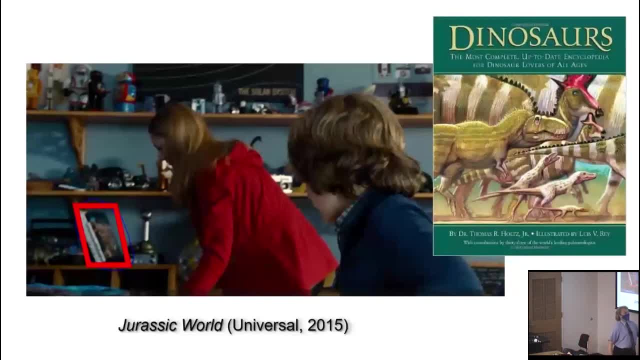 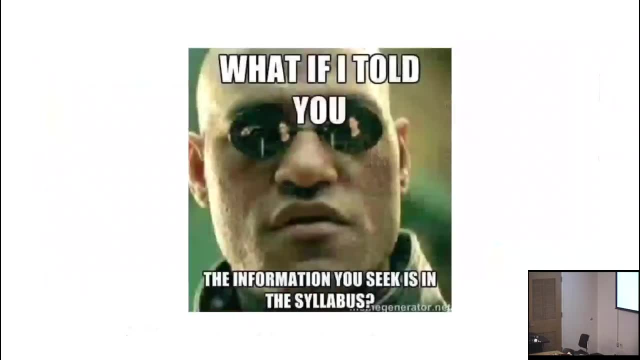 I thought I'm just fooling myself. You know that's not really my book, But when the Blu-ray came out someone was able to freeze frame it, And yet there it is. I may be really happy. 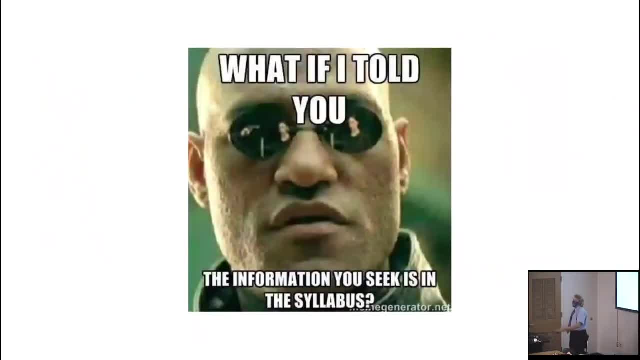 So, first lecture of every course, you'll walk through the syllabus. It's boring, It's dull. You just got to do it Because that's where the information is. So that's what we're going to do now. 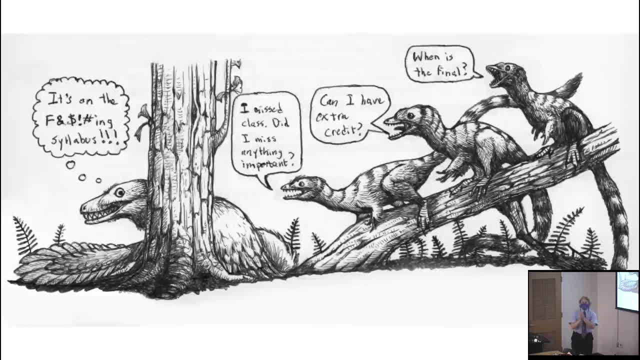 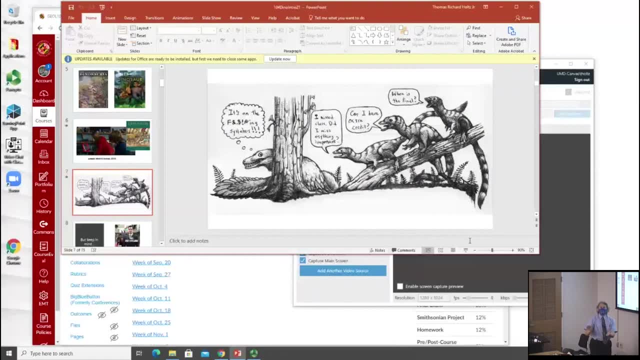 We're going to switch now to PowerPoint And I'll do the extremely exciting thing of walking through the syllabus Also. after decades of doing the dead tree variety of syllabi, the last year has convinced me. you know, I don't need to hand you papers. 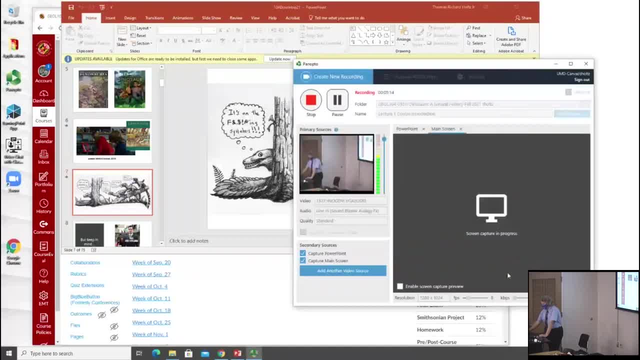 And so I'm not. I'm not doing that. Okay, it's claims. Oh, let's see. Okay, it is doing it. I don't need to burn that extra stuff there, Okay. So if you go to the ELMS page, 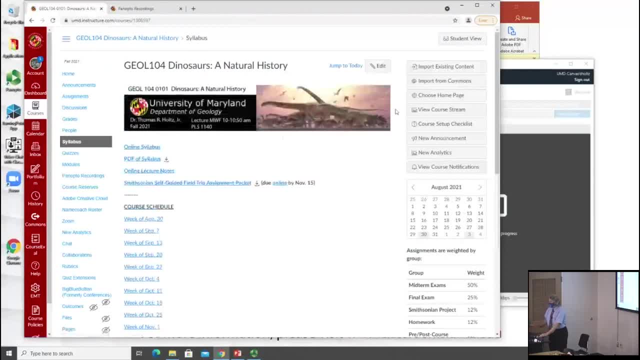 And I'm sorry I don't see student view here anymore. The interface on Canvas for faculty members is actually slightly different than the interface for students, So some of the stuff that shows up here might be like you would see. these things would be crossed out eyes. 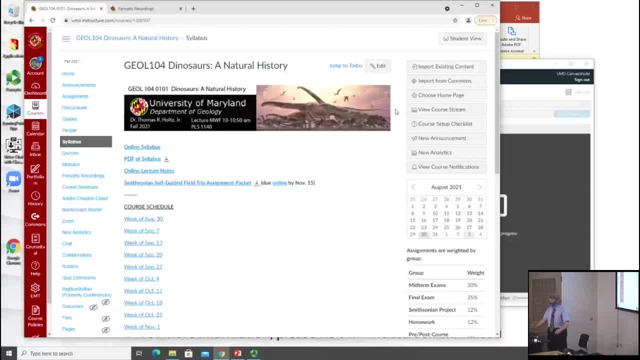 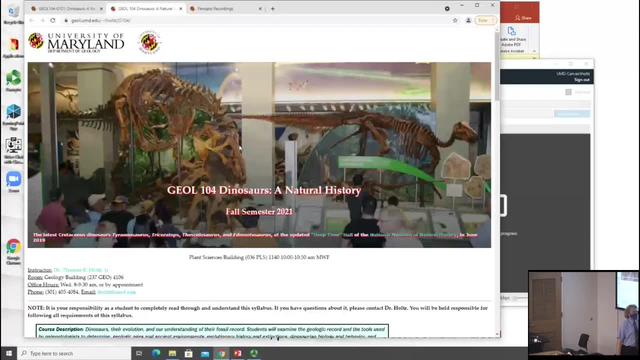 But in general it looks the same. So you can get to the syllabus from here, And so we're going over there. You can also get to it straight from the internet. Here it is, So let's walk our way through here. 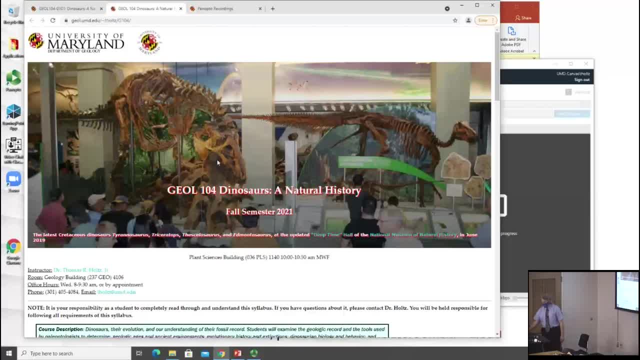 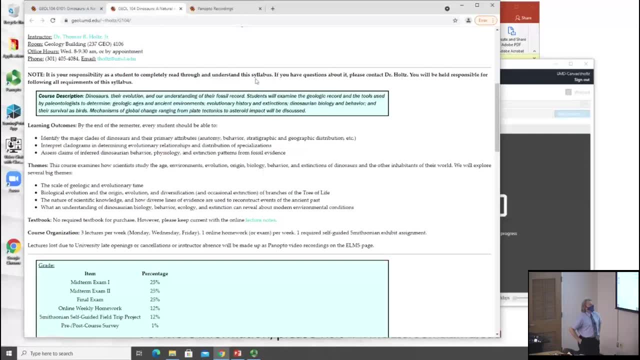 Super exciting. I know I'm going to skim over some of this because I'll get back to that moment here. I've talked about office hours. You know you can reach me here, Although using the ELMS inbox is probably the best way. 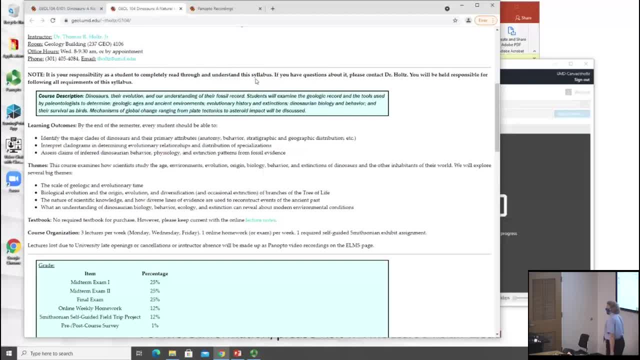 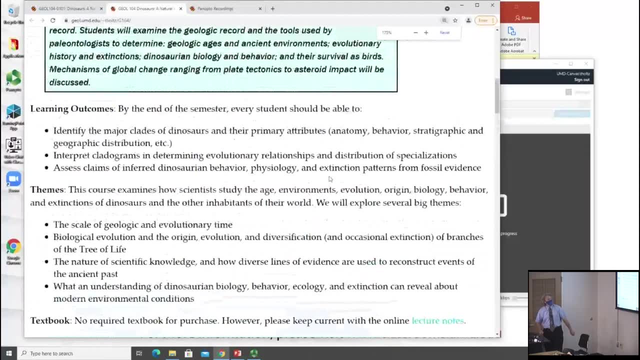 Those are super small books, Little print, isn't it? Let me bump up the print size. Let's see, There we go. That's probably better Learning outcomes. we'll talk about later Themes. we'll talk about later Textbook. 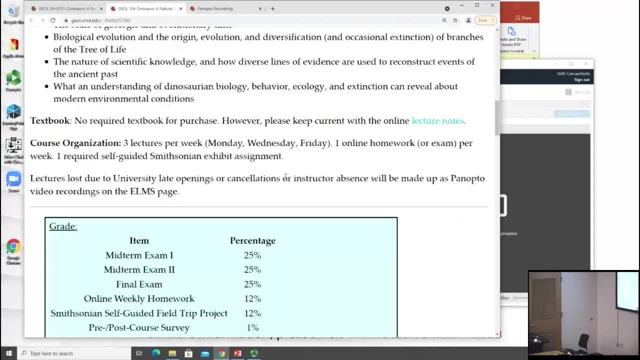 No textbook, No textbook can be up-to-date enough for this course. Information is always changing, Indeed, just point of pride, point of information. I've got colleagues around the world who use these web. notes that I do because they are the most up-to-date ones, because I update it every year. 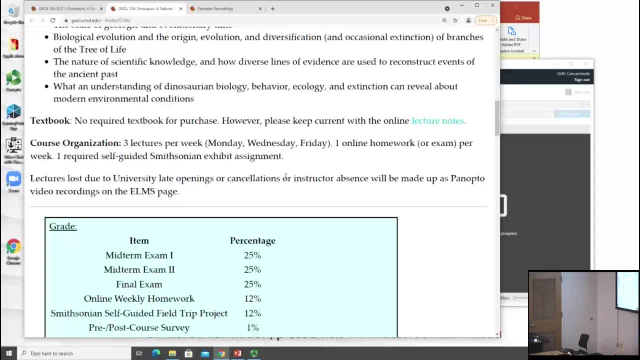 And, believe it or not, it changes, even though these guys are all dead. Course organization: Three in-person live lectures a week. Oh my God, This used to be so normal, And yet I'm freaked out by this. 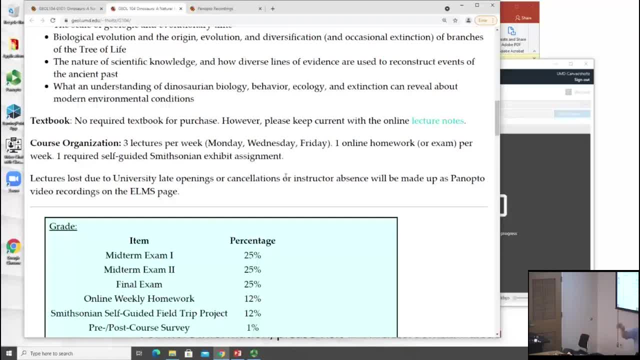 It's just weird. Our last lecture was March 20th or whatever of 2020. in person, I can actually stand and walk around. I can get my steps in lecturing again, So my name's not superimposed right here. 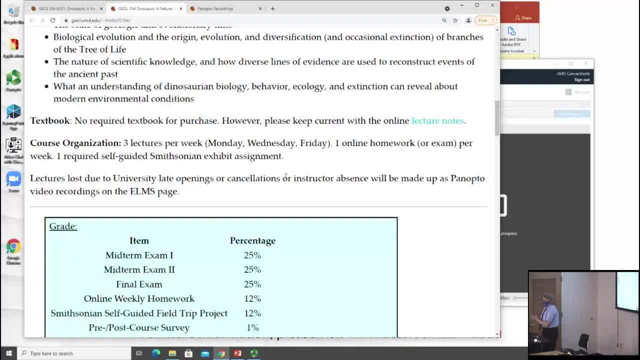 I can see your faces. It's cool. So each week there's generally some online homework or for exam weeks and exams. that's typically due on Friday. This week is actually a survey. Some of you have already begun to do that, which is cool. 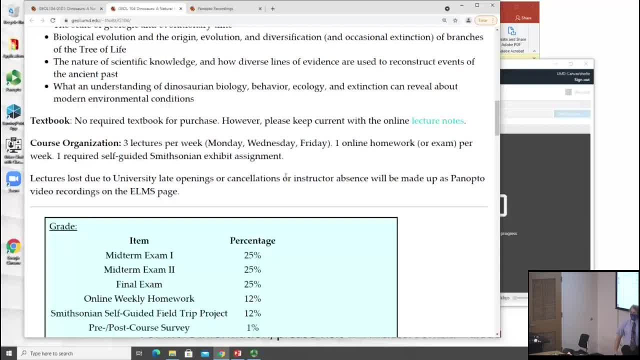 It's a pre-course knowledge survey. Next week it'll start to actually be worth Points based on how well your actual answers The survey. you do it, you get the full credit. You don't do it, you get zero. 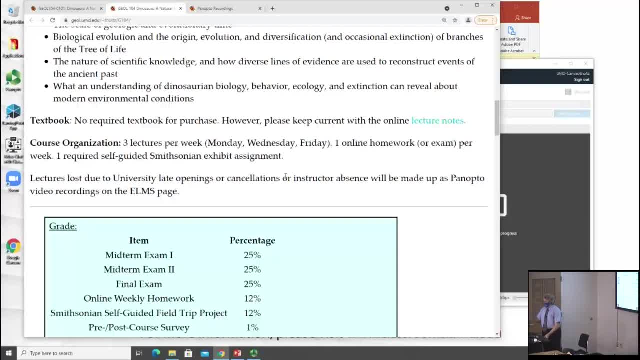 That's simple enough. Weeks of exams- I don't have homeworks- And assuming things don't get worse down with Delta, there is going to be a self-guided Smithsonian trip that each of you will go on. that's worth a grade. 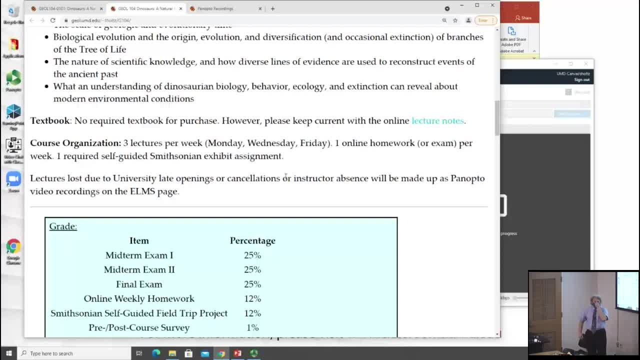 More detail on that later. More detail on that to come, although I believe you might be able to see the assignment right now. It involves going down to the Smithsonian, which currently is open. You don't have to have timed entry or anything. 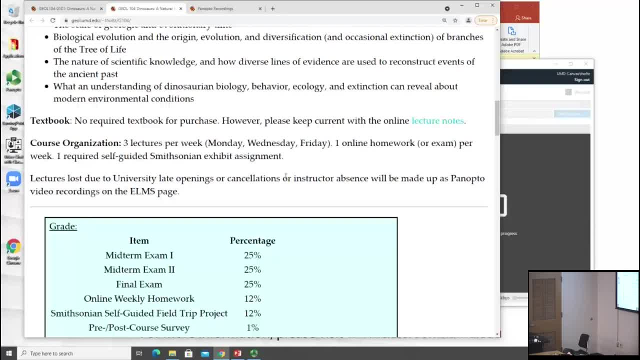 It's free And it walks you through the paleo halls and you answer questions based on your observations. You can do it in a group, but your answers have to be your own And if you go as a group, there are some questions that are pertinent. 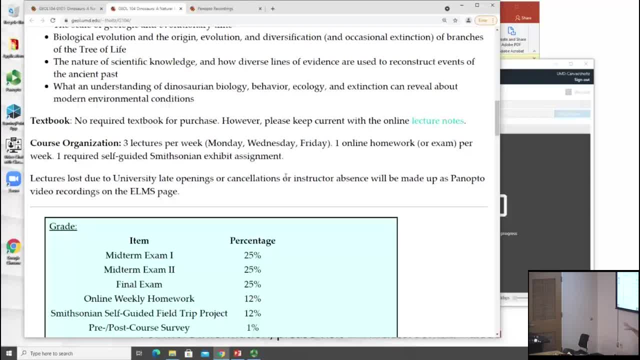 There are some instructions that are pertinent to that, like whether there's a bunch of options or things you could do. You're supposed to. You're supposed to choose a different option. Has anyone here seen these Smithsonian paleo halls since June of 2019?? 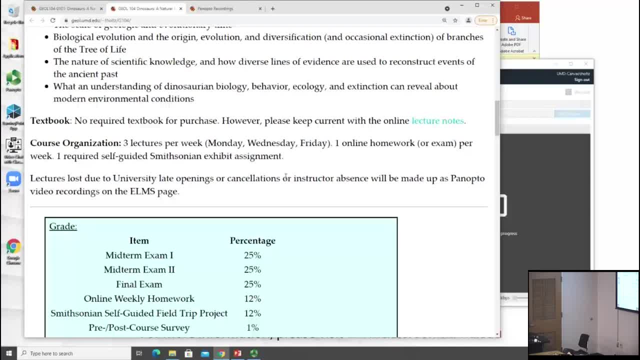 Okay, some of you have. That's awesome. There was a huge, huge reconstruction of the whole thing. It burned it to the brim, They took it to the ground, They built it back up. It's one of the most up-to-date exhibits in the world. 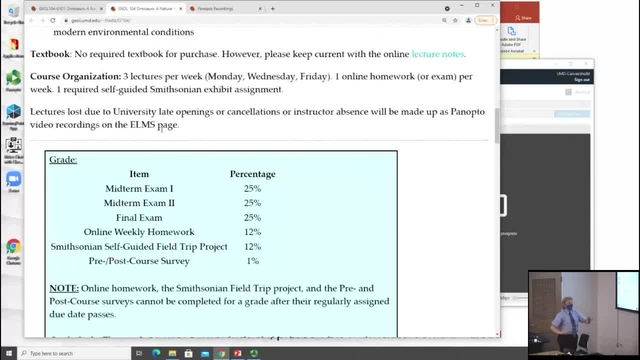 Let's take a look. Lectures lost to university, late openings: Did such happen? Not so much this semester. It's typically not that bad in the spring For the freshmen, By the way. she's like freshmen. welcome to the University of Maryland. 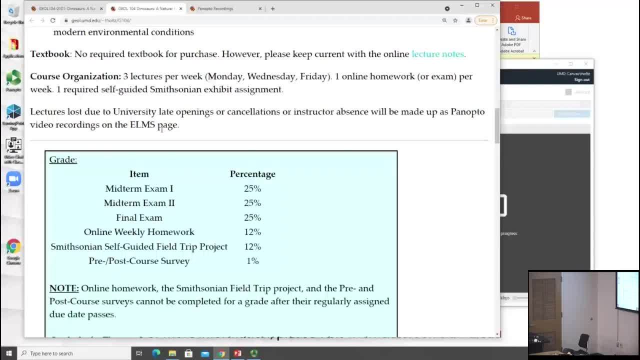 The freshmen don't necessarily know this, but the rest of you do. Spring is normally where we have late openings. If we have a late opening, I'll just record it on Panopto and we'll stay up to date, Or if I'm absent for some reason, 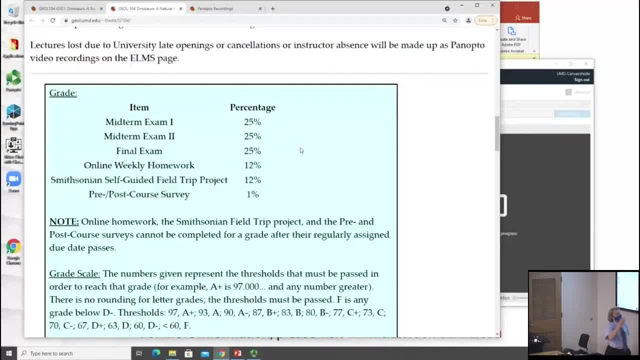 So just looking at the breakdown of the assignments: Exams are a quarter of the grade each. They're online, They're timed but open note. So an online weekly homework. as I mentioned, There's a self-guided field trip project. 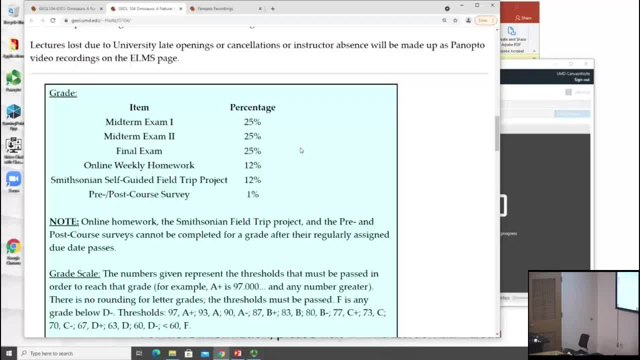 And then the pre-survey and the post-course survey. With regards to that- the pre- or post-course survey- I'm asking you to not use any notes. The idea is to dump the information out of your head. as you currently understand it. 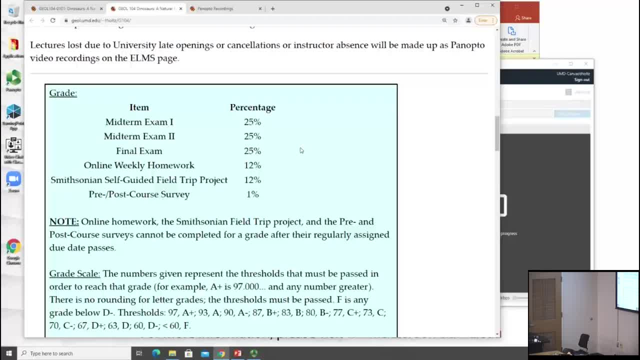 It is timed And the idea is to get a sense of how much of this information you know now, So that you can take the same survey essentially at the end of the course And I can see, hopefully, that you've learned something. 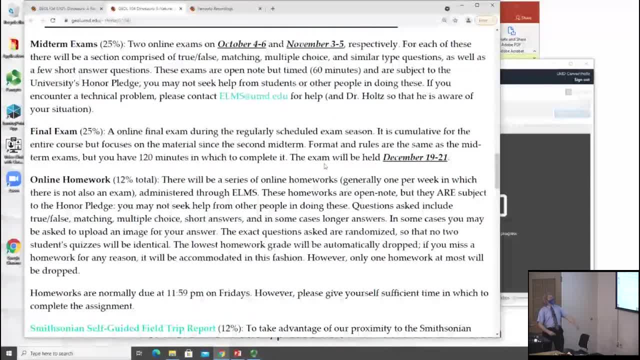 Okay, Midterms. There's the dates of the midterms. You've got several days in which you can do them, But once you start them, they're timed. They're subject to the honor of the university. They're subject to the honors pledge. 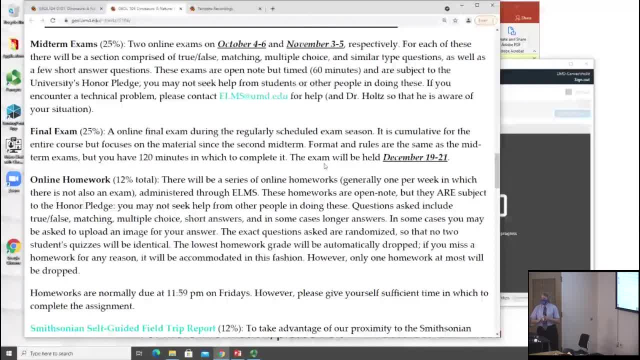 So you can use your notes, But you can't seek outside help from other people, Online homework. More about that when it gets closer Again. they're not also opened up, They're not timed. So those ones, once you know. 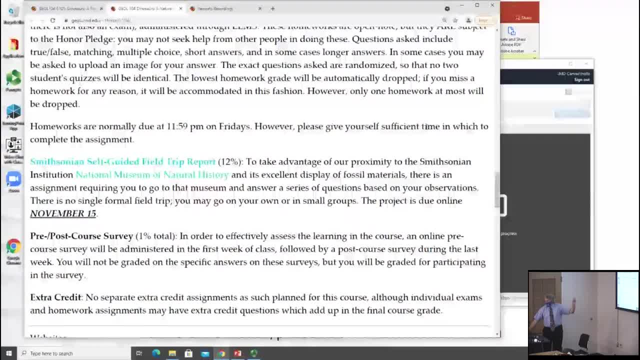 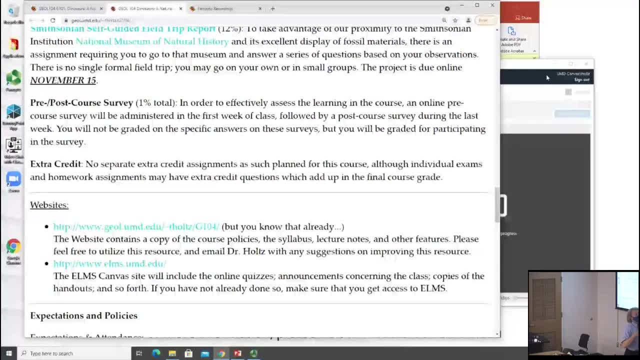 When you submit. that's when they're submitted. Field trip Survey. No separate extra credit assignments are planned for this course, But each of the assignments will have some extra credit, So it is entirely possible to get greater than 100% in this class. 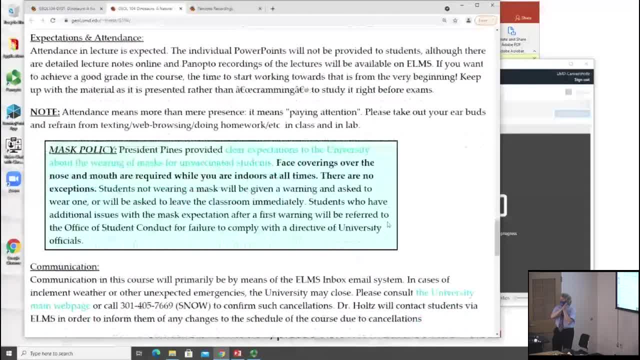 Websites. You know that. Okay, Attendance to lecture is expected. I'm not grading it, But it's expected. I say the individual PowerPoints about to provide it. That's technically true, But there's detailed lecture notes online. I'll show those in a bit. 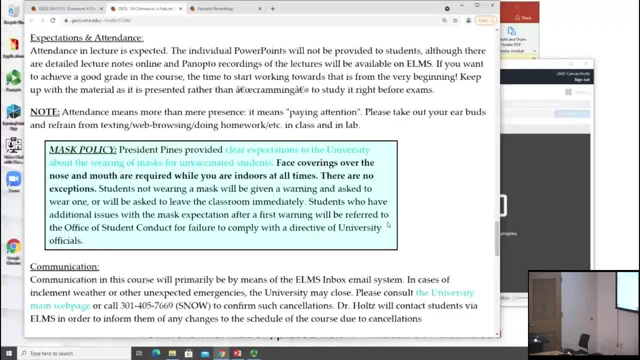 And Panopto recordings will be available on ELLs. If you wanted to have a good grade, that's fine. If you wanted to have a good grade in the course, we'll talk more about this Time to start working towards that from the beginning. 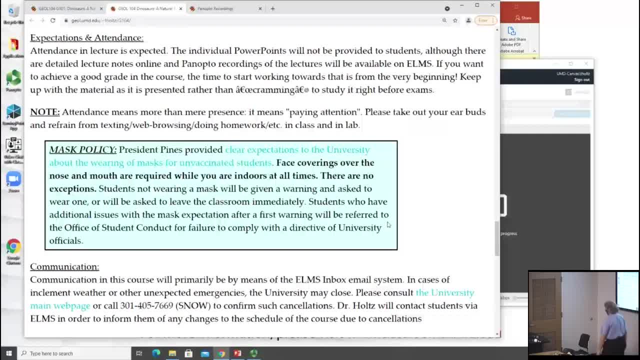 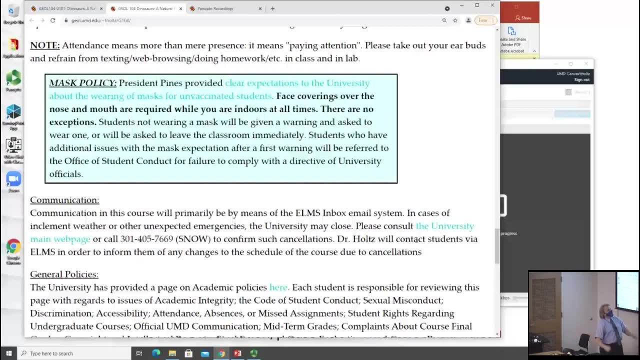 And bad HTML here. This is not some sort of weird language. I had curly quotes in the text file And you can't do that in HTML. Okay, By the way, attendance is more than your presence. It's actually paying attention. 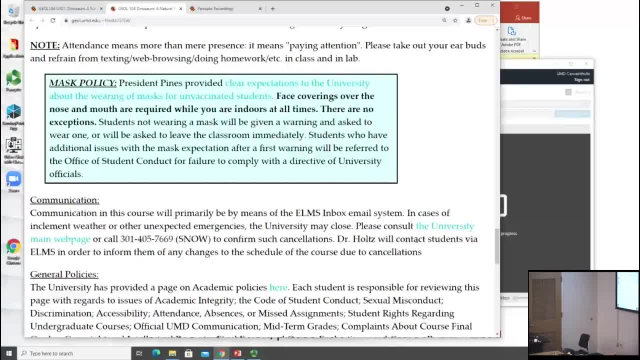 So try to take out your earbuds and refrain from non-relevant class stuff in class Or in lab. That's a cut and paste error. There's no lab Mask policy, Brand new. I even sent out an announcement about this. 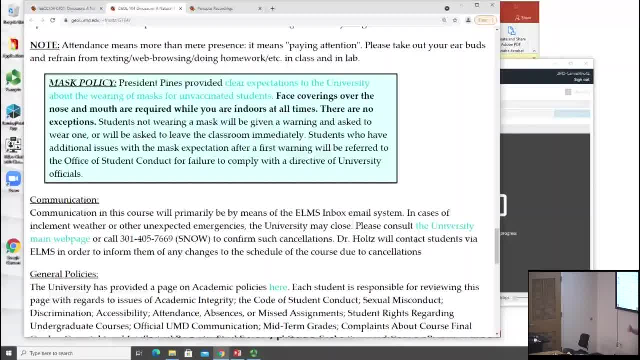 Cool, I'm going to have to say these words anyway, But it looks like it's not a problem. So Expectation Said: not over the summer, Everyone wears masks for the benefit of the unvaccinated And each other too. 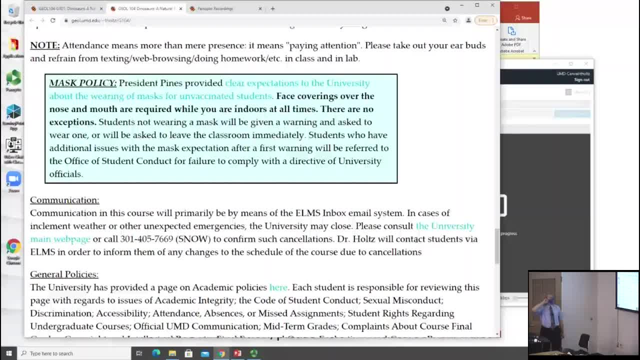 Because you know adults is nasty. Face coverings over the nose and mouth are required while you are indoors, at all times, And that's what we're going to talk about today: We're going to talk about face coverings. We're going to talk about face coverings. 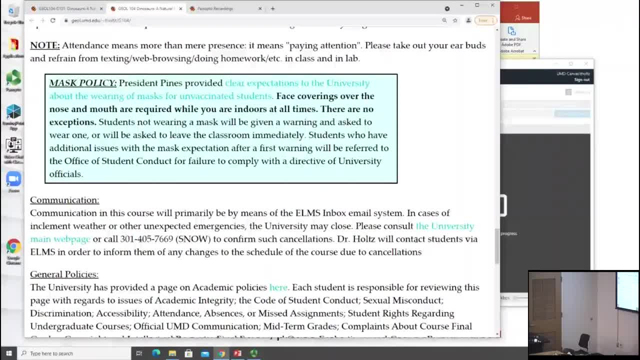 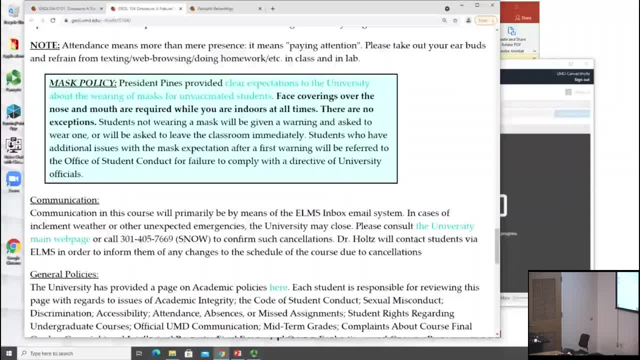 And asked to wear one. If you choose not to do so, You will be asked to leave the classroom immediately. Students who have additional issues with the masks expectation of their first morning will be referred to the Office of Legislation of student conduct or a failure. 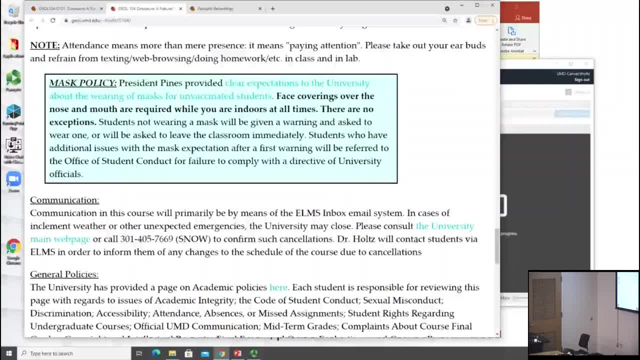 to follow a directive of the university. Okay, I've done my job. I was supposed to say that, Hopefully I'll never have to do it again, And you won't either, because this is for your benefit Also, by the way. 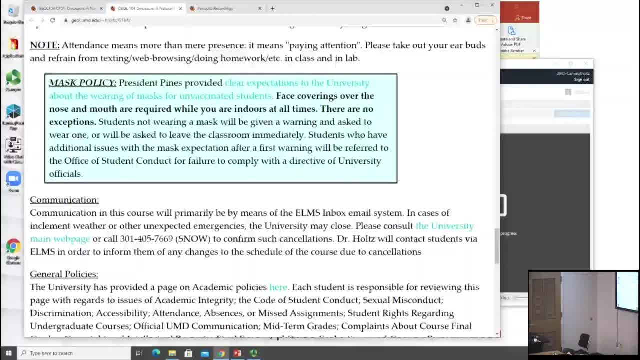 in the back row. can you hear me clearly? Awesome, Technically speaking, the university would allow me not to wear the mask during lectures if I'm more than six feet away from you. I would consider that a dick move if I was able to go without a mask and you guys had to have. 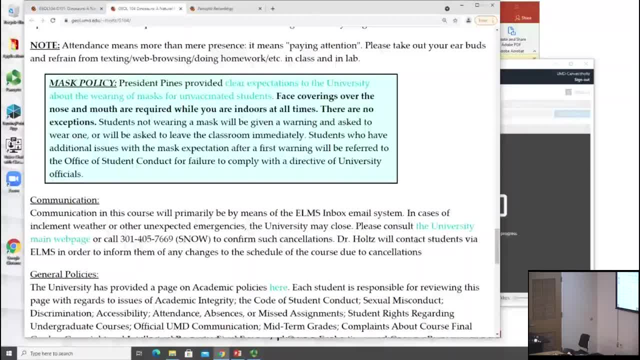 one. So my intention was to wear a mask, but if you couldn't understand me then I might have to rethink that. policy: Communication: Use inbox for anything. Policies: I'll talk more about those in a bit. Laptop policies: 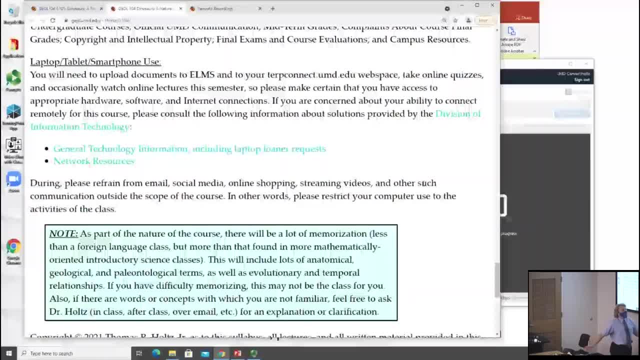 You've got to be able to use ELMS for this course. That's where the quizzes are, etc. So if you need additional information or initial help like load a laptop- say, one of yours breaks down- or if you have one, 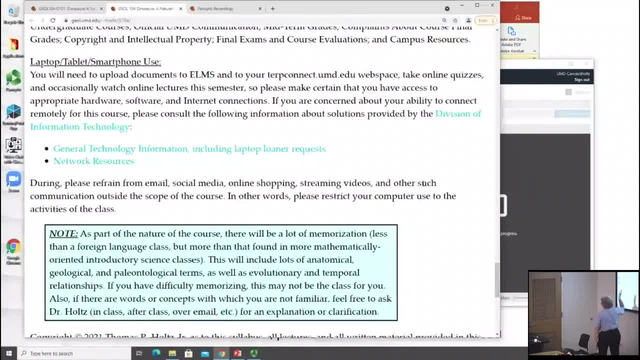 and it breaks down. or you need good networking and you don't have it yet. the university is here to help you. You're not paying a heck of a lot of money to go here. Use the resources that they provide. Note as part of: 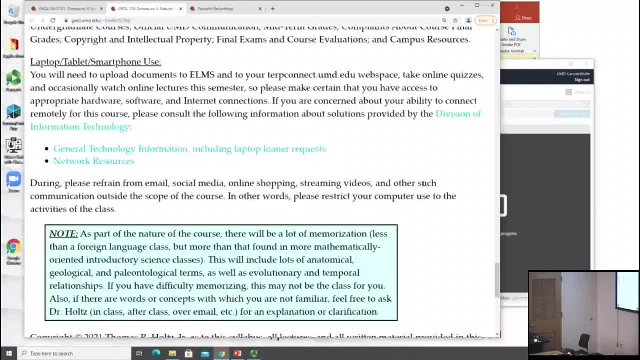 this course there's a lot of memorization. It simply can't be helped Less than in a foreign language class, but more than more mathematically oriented pro-science classes. So terminology from anatomy, from geology, from paleontology. 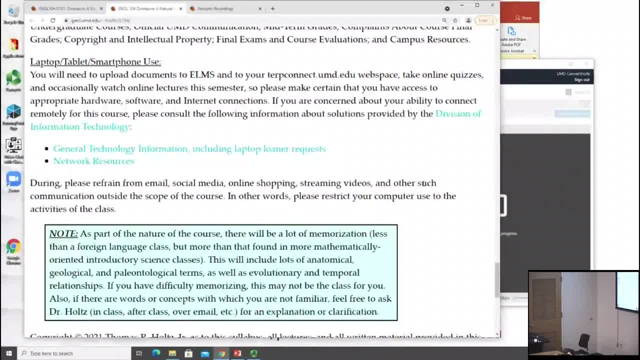 from evolutionary biology and so forth. Honest to goodness, if you know already that you have difficulty memorizing terms, then honestly this is probably not the course for you. And just saying that up front, Because you are expected to know that And know what the 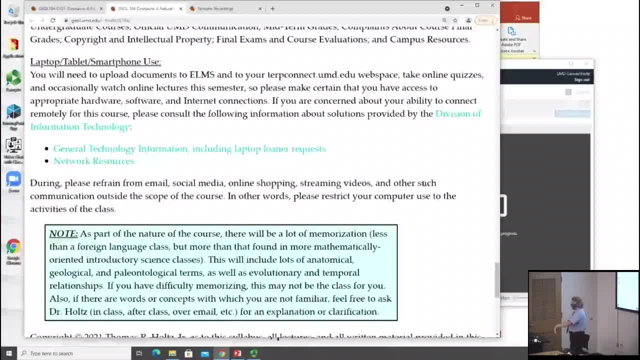 distinction is between a ceratopsian and a neoceratopsian, A ceratopsian and a ceratopsid, and so forth. You're not expected to know that yet, But you will be later on. So also if you have questions about words. 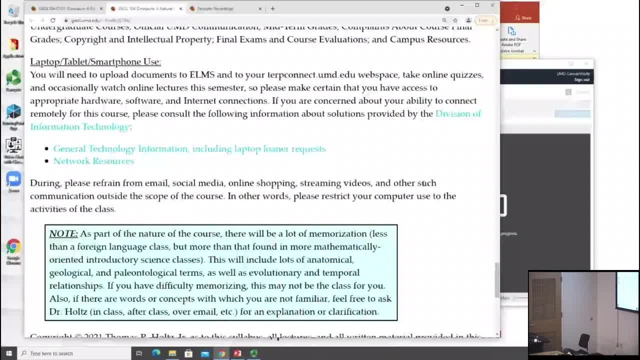 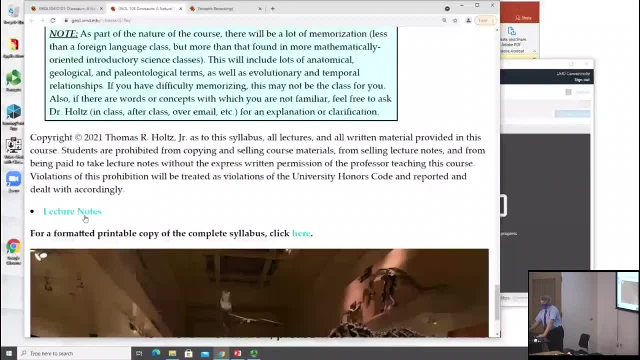 or concepts that you're not familiar with, feel free to ask me in class or after class or over email or whatever, and we'll clarify it. Okay, the lecture notes Go over here. So I provide lecture notes. They're not a script. 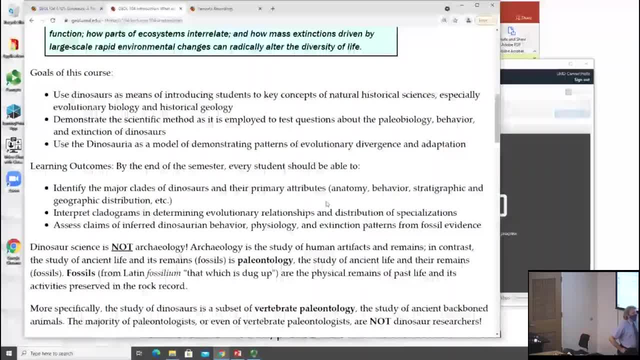 They're not exactly what all that I'm saying word for word. It covers the key concepts. It actually covers more than anything I might say in class typically, Sometimes a little less, but generally it's got more detail than I'll say in class. 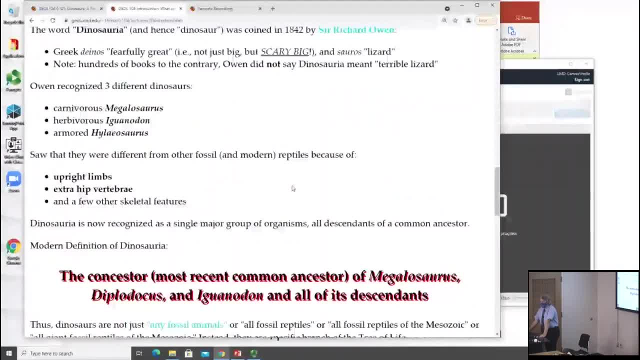 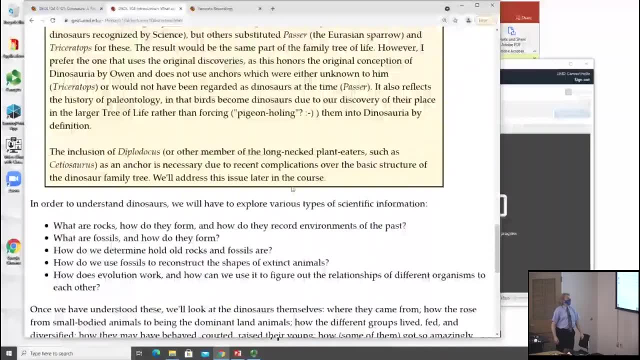 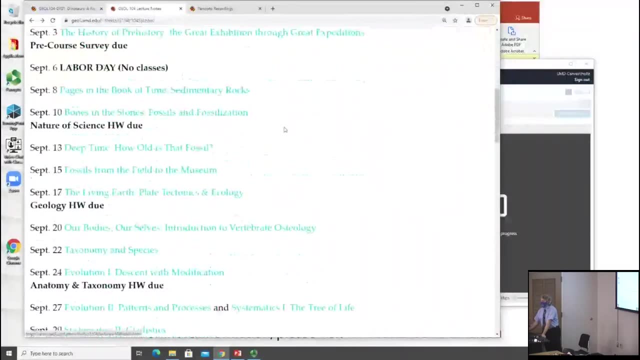 They're an important resource. You should go to them to read them in detail. You can follow along and so forth, but it's sort of good to watch the PowerPoints and then check these out later, And it's listed in the order that we do this. 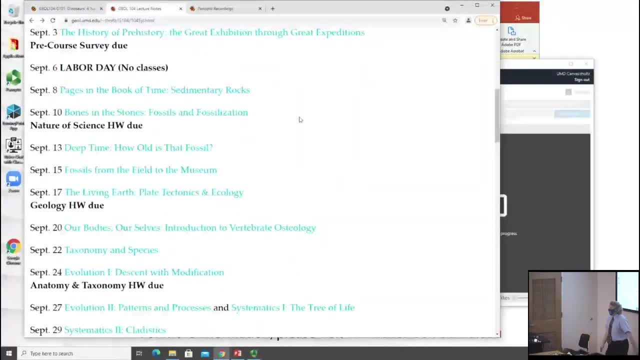 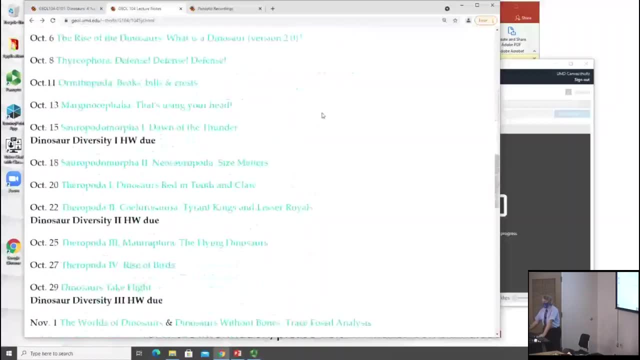 By the way, of course, a week from today we don't meet because it's Labor Day. We actually have like holidays this year. That means something, So you know later on we got things like this and there'll be information. 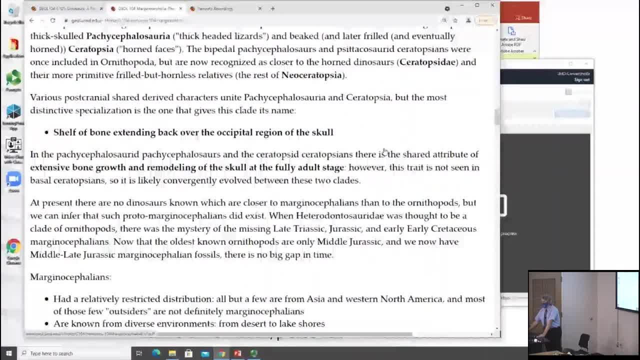 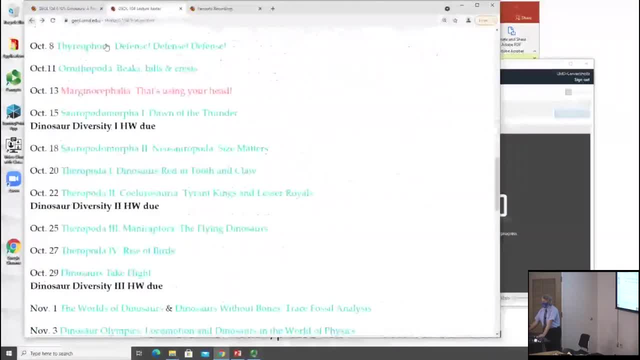 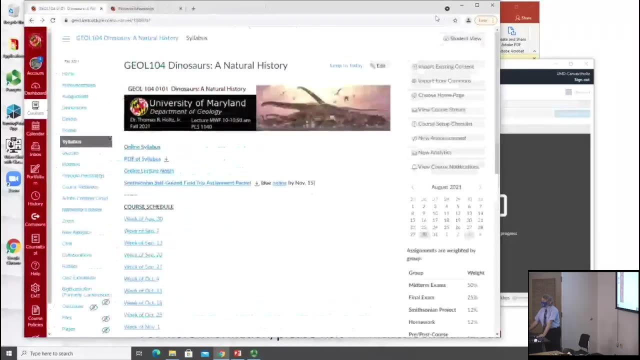 like cladograms and more cladograms and details and so forth. Often there's like links to pictures and so forth. So all right, So far, so good. Awesome, All right. so let's get back to the PowerPoint proper. 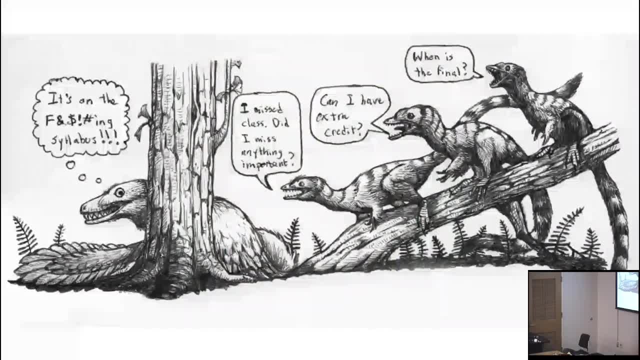 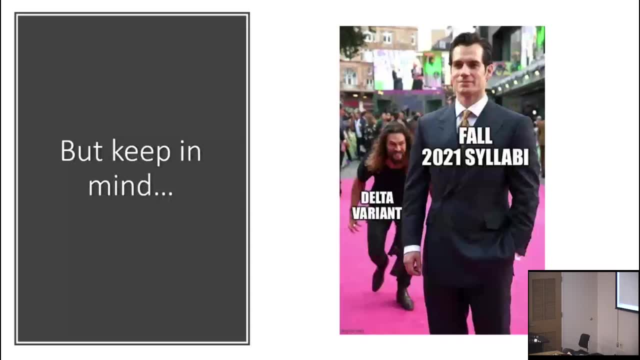 And in fact I'm gonna duplicate some of the stuff that I had already said, so I'll just skim through that And keep in mind. you know, I really want to be able to get through this semester and this school year. 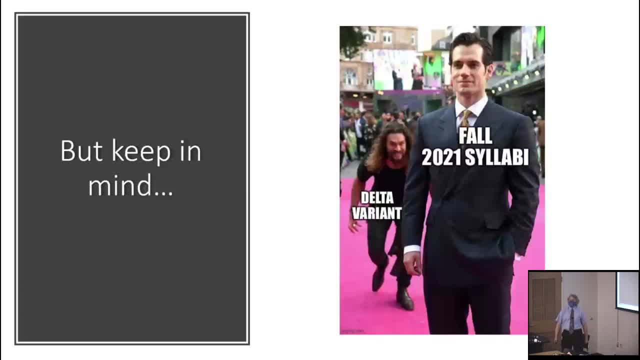 in person, maybe even, who knows, maybe even by the spring, to be able to do this without a mask. we'll see, But it's lurking in the background. so And other ones. Course website. I already went through this. 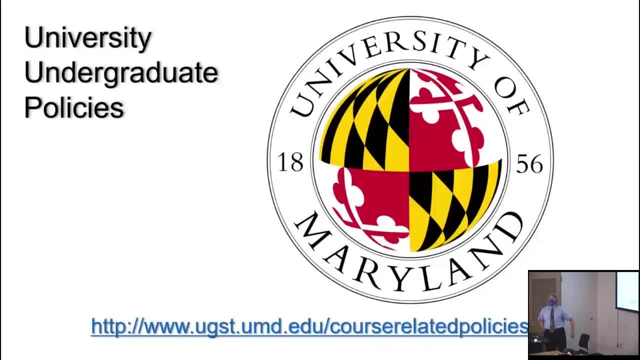 Undergraduate policies. I'm not gonna go through this in detail. If you're a freshman or if you're an upperclassman and haven't checked this out yet, there's a single website that the university has provided where basically course-related policies are there. 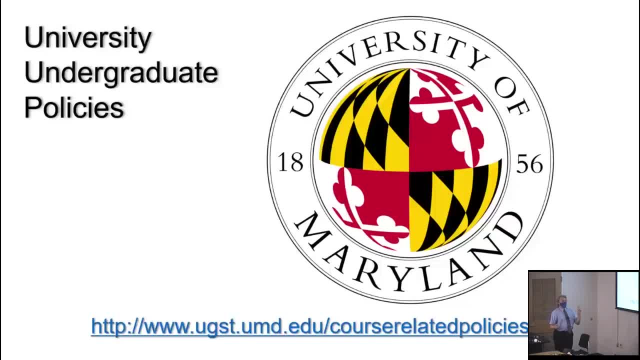 These include things like the Honor Code, and if you see unfair grading, you know heaven forfend, but you know harassment, all sorts of things like that Excused absences. It's worth having a check out at this. 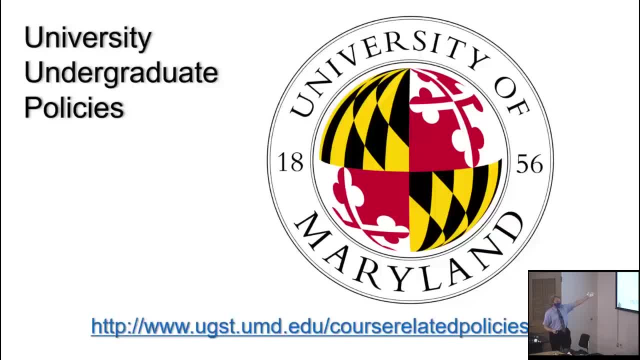 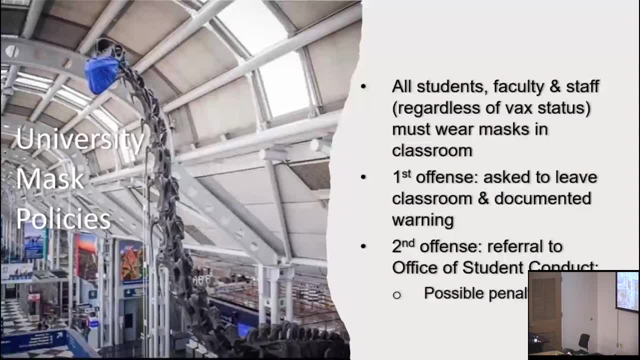 if you haven't already seen this, but I'm not gonna belabor it- just making sure that you're aware You've got protection and you've got responsibilities, Mass policies- I already mentioned this, By the way, too. you know you can help each other with it. 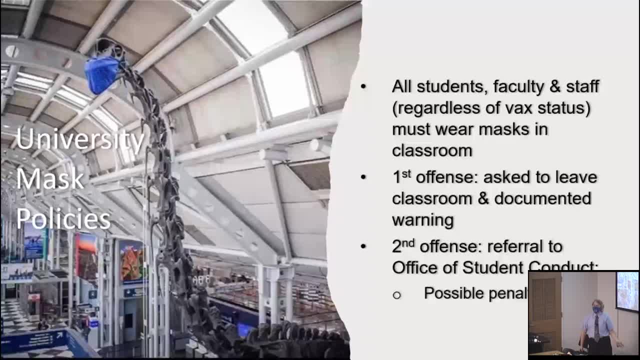 I guarantee at least one of us is, and it could include me. that's why I'm saying us might forget to wear a mask when we come in. so if you know one of your friends could nudge you and if my brain was working. 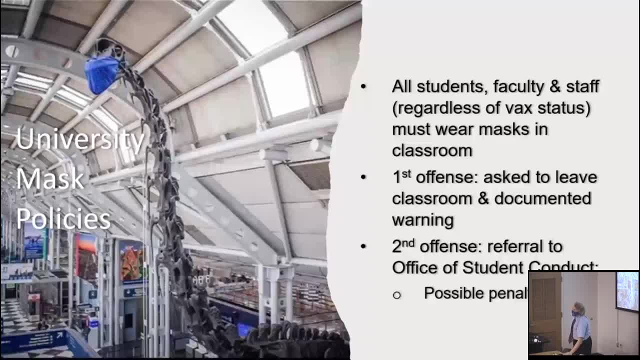 if I wasn't having a pandemic brain, I would have had some backup masks with me, Or I actually have one. So had there been someone who showed up without a mask, I would do that. oh, I want to bring in the disposable ones. 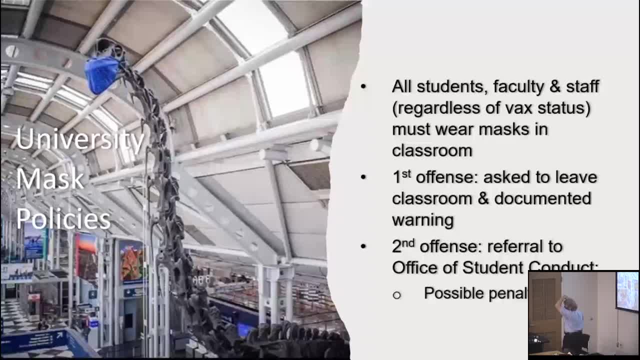 because I don't want to get rid of the ones with people. So you know we're all in this together. All right, The Brachiosaurus is doing it. Anyone here fly through O'Hare ever and see this Brachiosaurus? 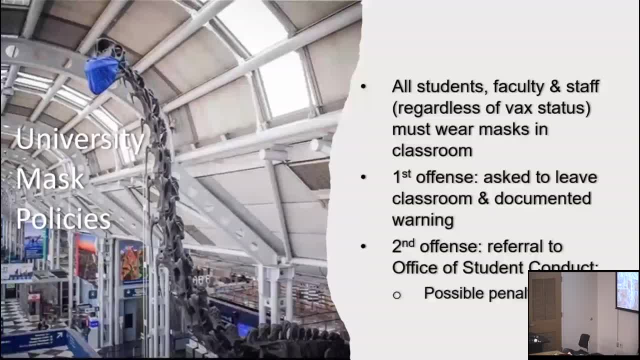 Yeah, it's. I think it's a Contours B, but it's a skeleton of one of the largest Jurassic dinosaurs in North America that the actual specimen is at the Field Museum in Chicago, but they made a cast. a lot of it is restored. 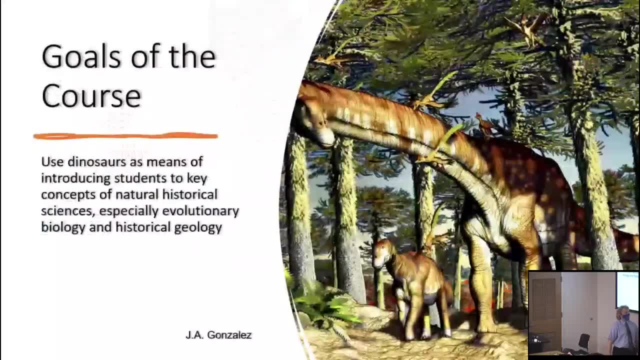 and it's hanging out in the airport. So goals of the course? Well, I have a course on dinosaurs. The goal here is not to train the next generation of paleontologists, because you have plenty of those, although some of you are interested in going on it, yay. 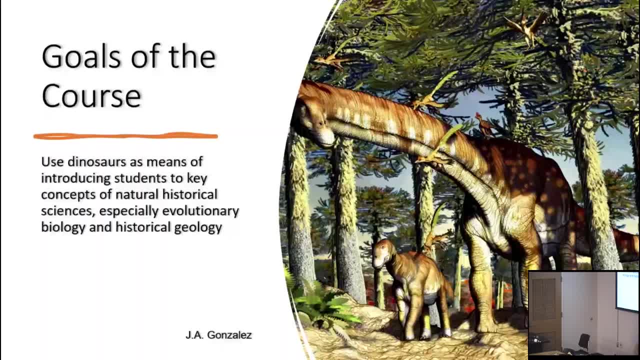 I will say that there are PhDs in the field currently practicing who've been through this course, But the goal is to use dinosaurs as a means of introducing students to key concepts of natural historical sciences, especially evolutionary biology and historical geology. 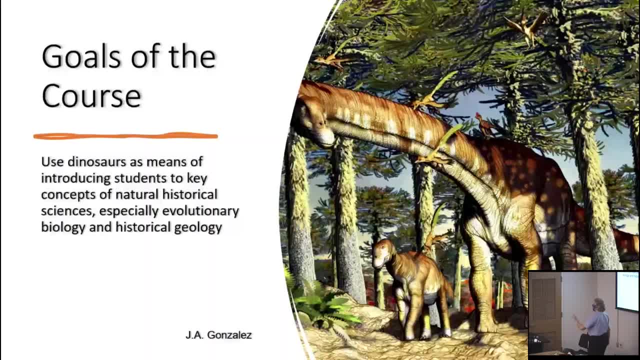 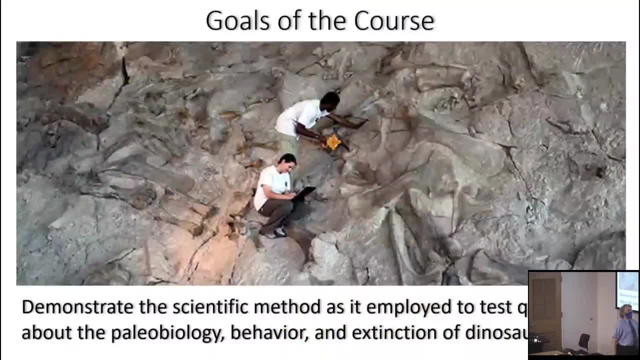 So dinosaurs will be the focus, but through them we'll talk about broader concepts in the natural historical sciences And so, even more broadly, to demonstrate how the scientific method is used in this case to test questions about the paleobiology behavior. 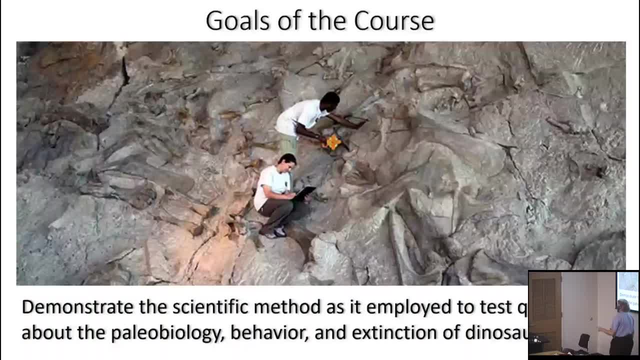 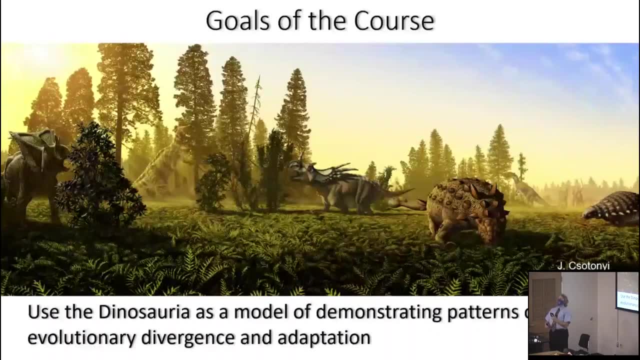 and extinction of dinosaurs. In fact, Wednesday's lecture is specifically about what is the scientific method. I'm noticing that clock is. I'm noticing that clock is. I'm noticing that clock is no bearing on any time relevant to. I gotta make sure I'm 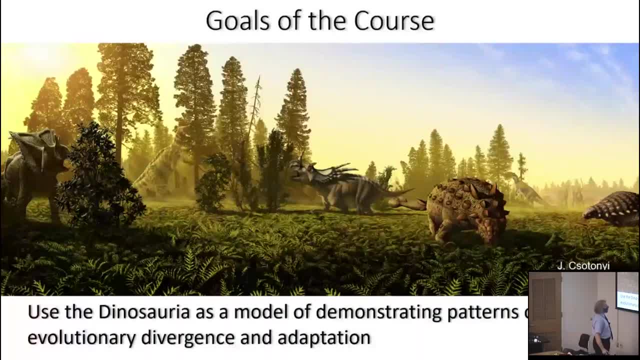 a little working to this, Okay. Another goal, of course, to use the dinosauria- that's a technical name for dinosaurs- as a model of demonstrating patterns of evolutionary divergence and adaptation. The middle of this course, specifically, is gonna take a walk through the family tree of dinosaurs. 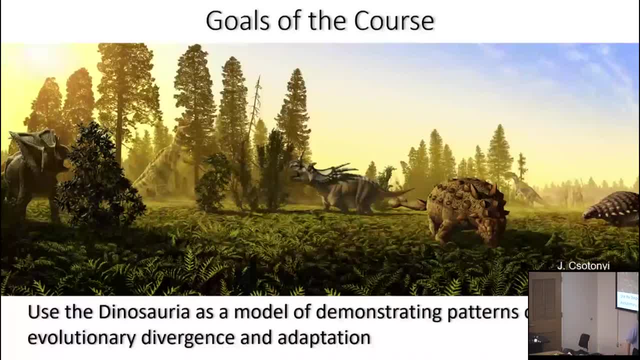 And up each branch we'll see their changing anatomy and ecology time And you know there'll be sort of lessons learned of these different pathways so you can get to learn these different dinosaurs. So a note about attendance. I already said attendance. They show up. 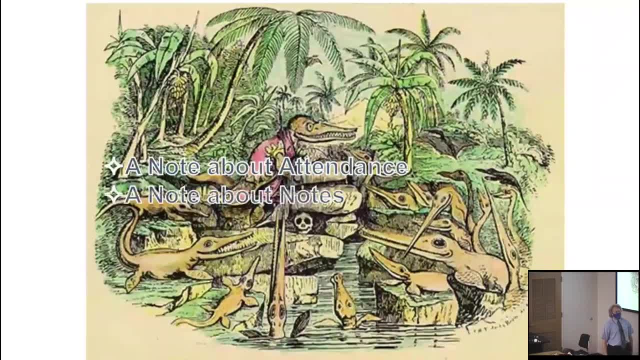 and you pay attention. A note about notes. The online notes are available, but I see some of you are writing down notes and that's awesome. Actually it's been, and some of you might be typing them too. It's been shown. 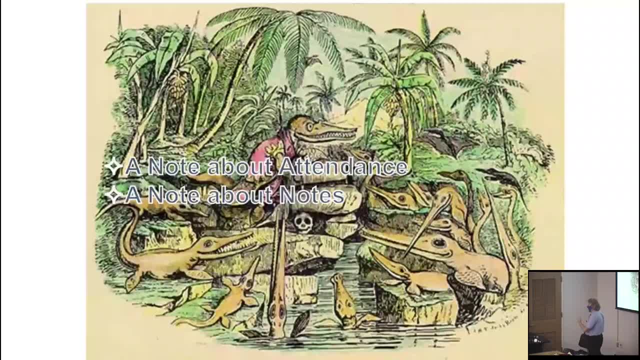 by experts in education. you know educational sciences that the act of taking notes actually improves your ability to understand the material Because you become an active learner at that point. and active learning, you're using different parts of your brain in that. 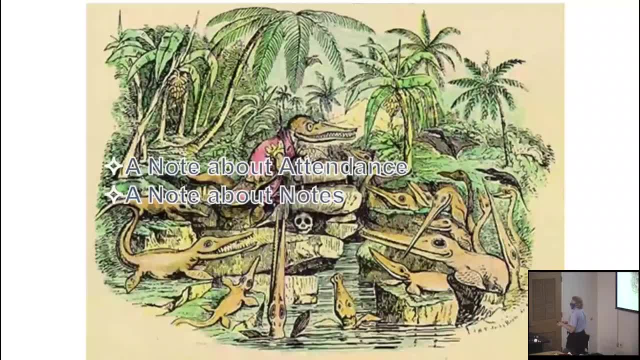 and you learn it better than simply passively. in general. Now, for some people it's good to go through a lecture and to sort of listen to it and then go back and maybe read the lecture notes and so forth. That'll help reinforce it. 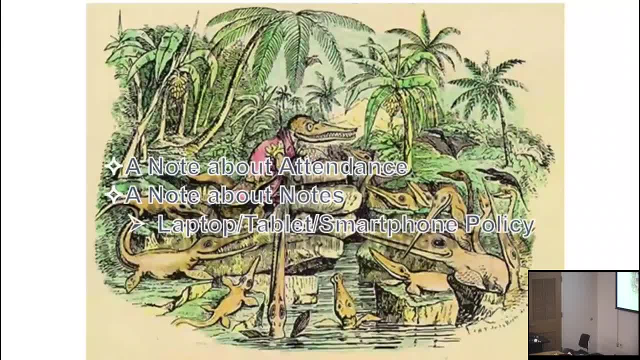 So towards that end. you know use of laptops, tablets and smartphones is fine as long as you're using in-course relevant stuff. You know, checking out social media at the time or doing work for other courses, However tempting that. 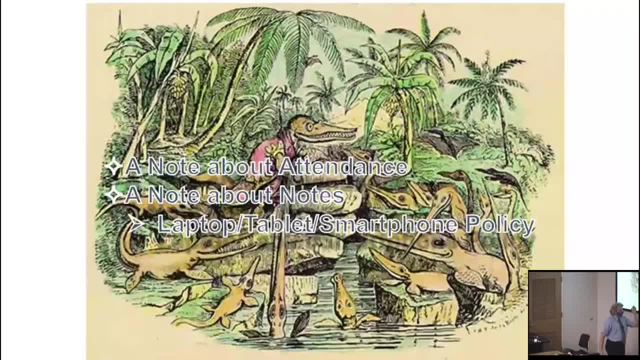 might be, it's not that helpful. And you know, honest to goodness, I get you know. this is not a bragging thing, this is a factual thing. I have 16.6 thousand followers on Twitter. I'm not. 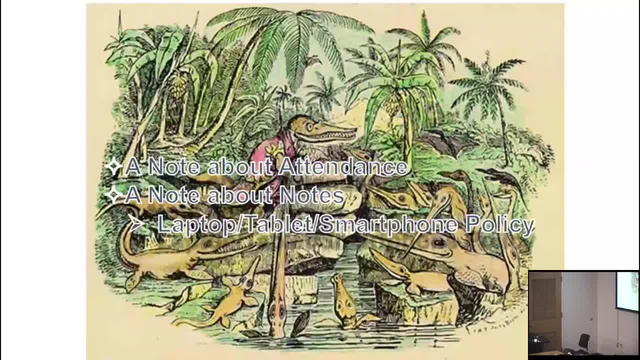 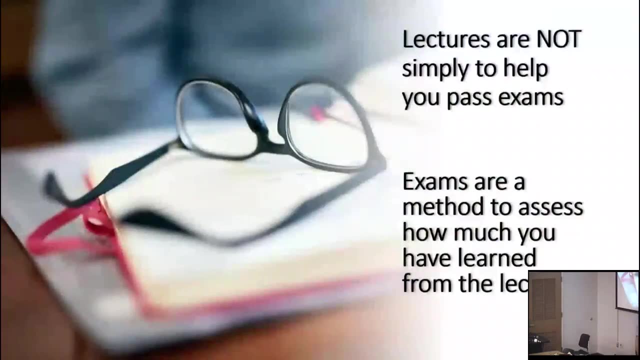 I am not familiar with social media, But during class I'm not like posting anything. So, yeah, Limit to following, taking notes and searching for relevant information. Now this next statement may seem bizarre to some people. 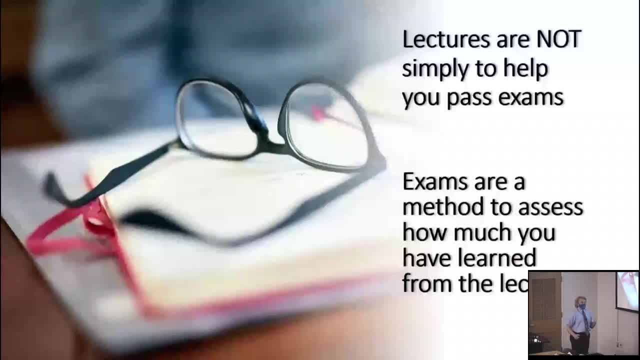 But it's actually true. Lectures- and, for that matter, homeworks- are not simply to help you pass exams. The goal of the course is not to pass an exam. This is not a course that's going to lead on to a technical certification. 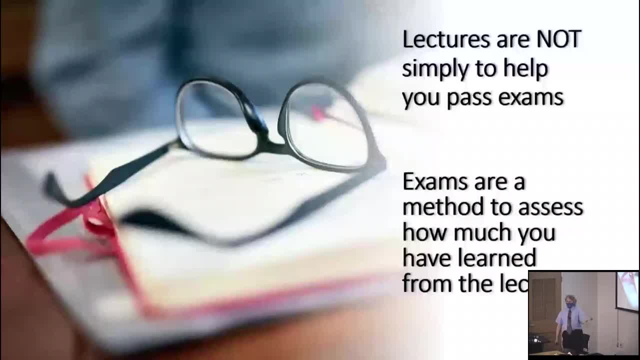 or anything like that. This is a course of information, And so the idea behind the exams. they're a method to assess how much you learn. So, believe it or not, because I get like course evaluations of, I will teach you things. 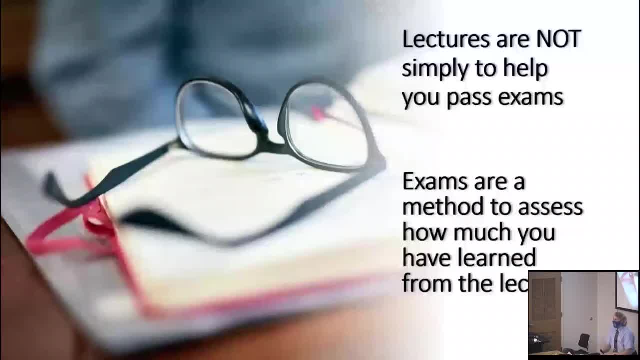 that never show up on the exam. I know some people go, oh my god, they'll complain. He taught us stuff And it never showed up on the exam. Yeah, First of all, if I taught, if I quiz and examined you, 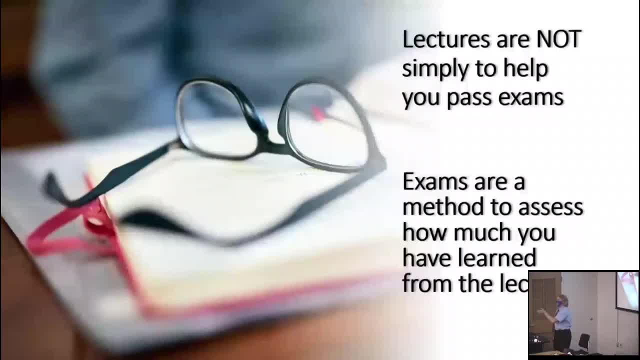 on everything that I taught you. it would take as long as the course. That's not going to happen. Do the math And the exams are just a way of seeing that you're learning the material. I know that's not the paradigm that some people learn. 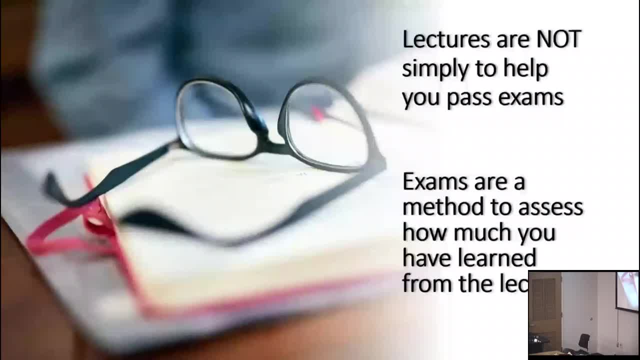 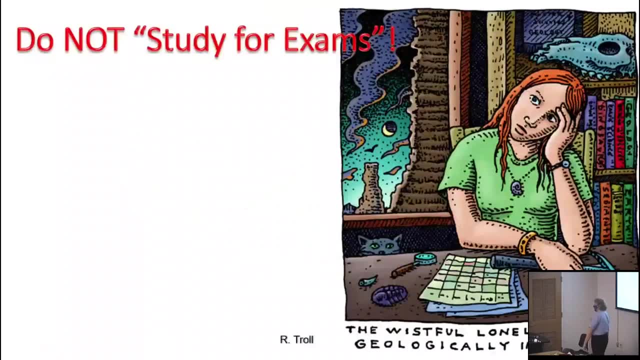 And I get it. But I just want to because I've had these complaints in the past. I wanted to say that up front so you can be thinking about that Towards that end. it's actually not super beneficial to specifically study for exams. 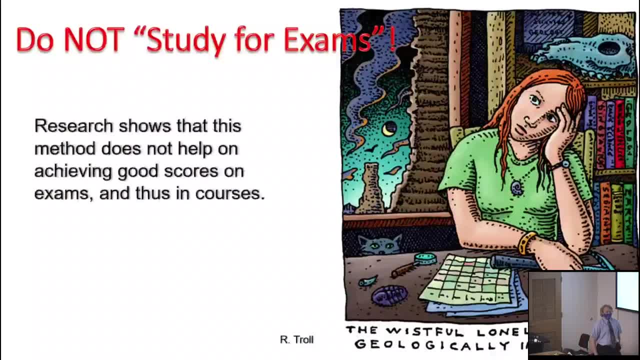 Now I want you to study, But research shows that sort of cramming for exams at the last minute doesn't actually help you achieve good grades And it certainly doesn't help you retain this information You know, basically dump it into short-term memory. 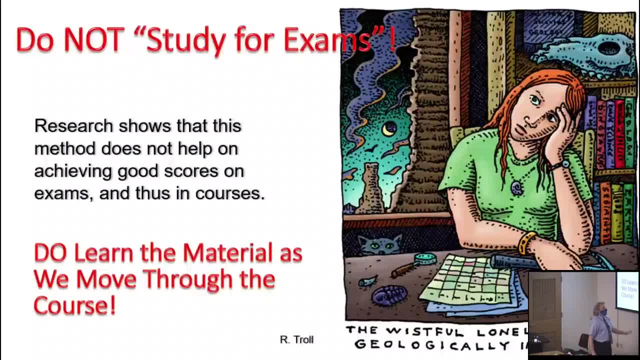 and then sort of evaporates. Basically it helps a lot more to learn the material as we go through the course And the more modalities you use talking about it with friends, you know, classmates or people who aren't in the class. 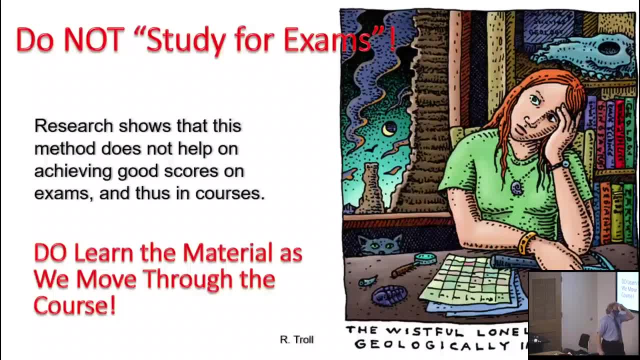 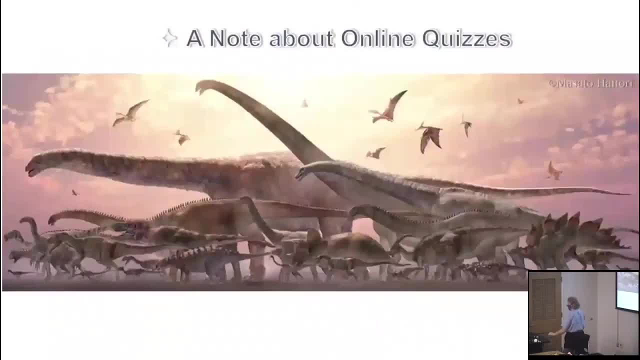 writing stuff down, whatever, then actually, because you're using different functions of the brain, you learn it better and you can recall it and you can synthesize it, Know that online- I should say online homework, So I'm calling them homeworks this year. 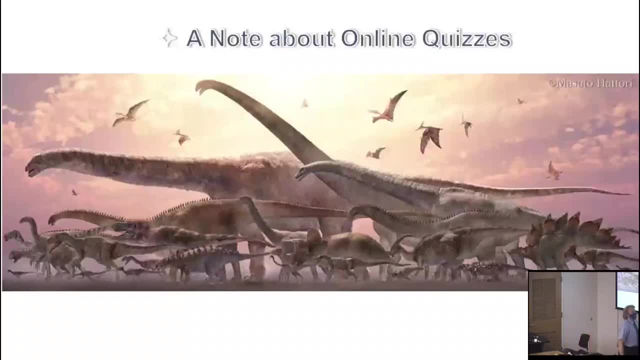 although they're really quizzes for the most part. Okay, They're online. as I said, They'll be available typically early in the week. they're due. They're due Friday evening. They're done on L's. They are not timed. 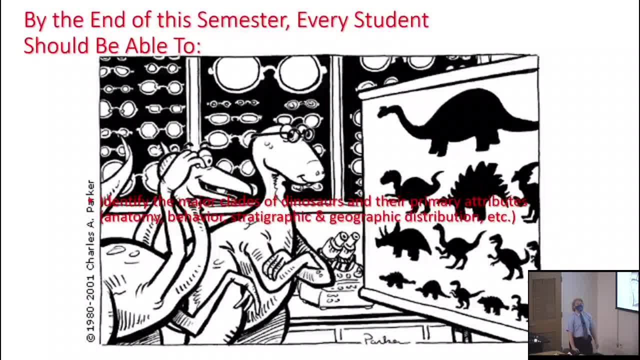 Okay, Of course, learning outcomes. We're supposed to identify specific learning Outcomes for classes, So by the end of the semester, every student should be able to identify the major clades. What's a clade? All right, we'll get there. 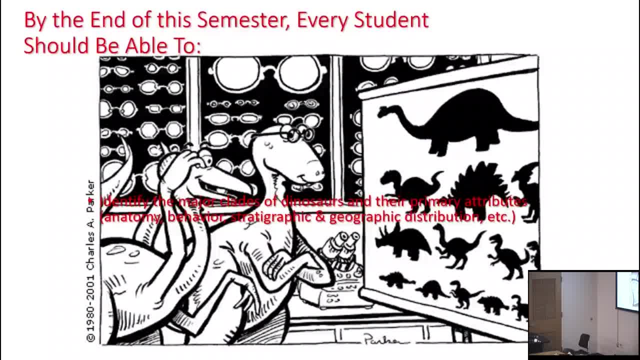 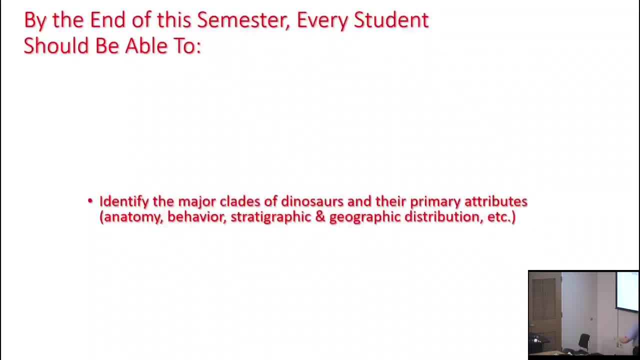 A branch or part of the tree of life Clades of dinosaurs and their primary attributes, Those things like their anatomy, their behavior, stratigraphic- that's, time and geographic space distribution, et cetera, So that you would be able to recognize. 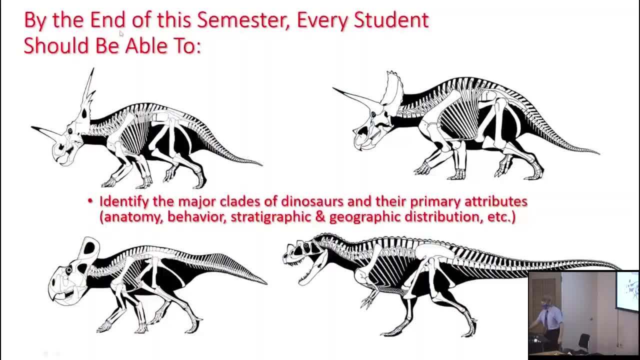 a- let me do this here so it shows up on the video- A, a ceratosaur, a neoceratopsian, a centrosaurine and a ceratopsian, which are both ceratopsids. 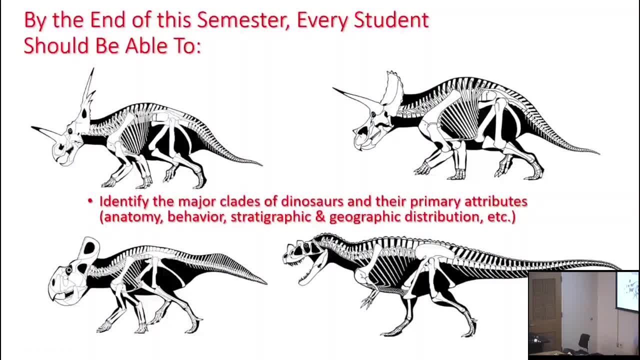 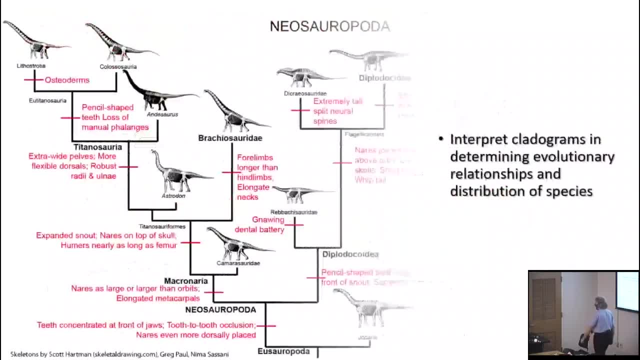 from each other. I know it's scary. now Don't worry. That's why marching up the tree of life will be very helpful. Okay, To be able to interpret cladograms. the cladogram is one of these thingies: The branching family tree. 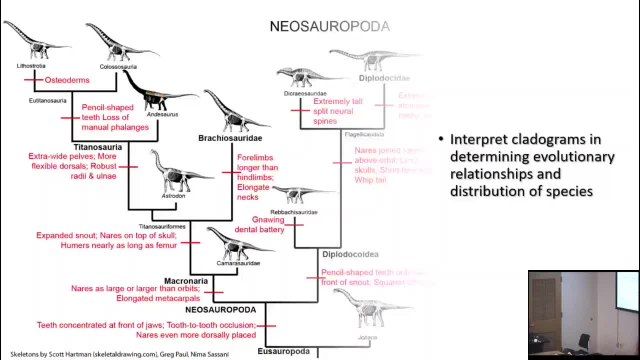 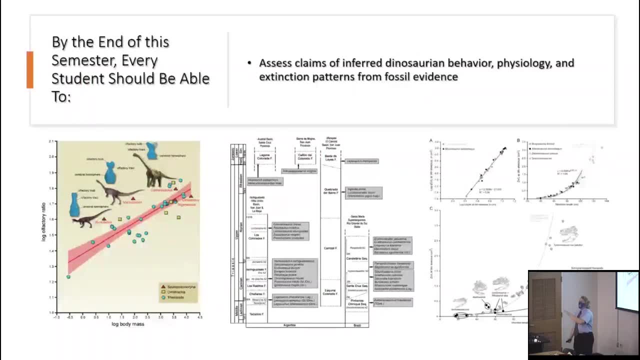 In determining evolutionary relationships and the distribution of speech and the distribution of species and, for that matter, the distribution of traits. You're not expected to know this in advance. If you knew all this in advance, you wouldn't have to take the class. 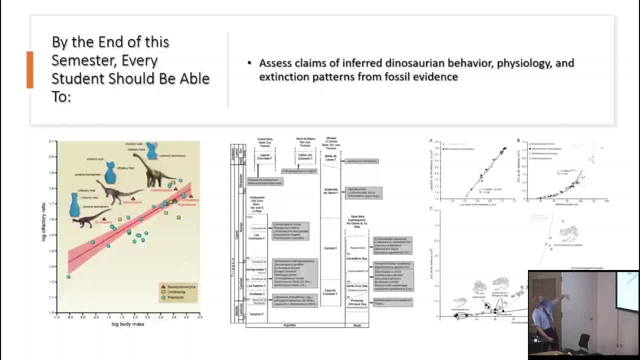 By the end of the semester everyone should be able to assess claims of inferred dinosaurian behavior, physiology, extinction patterns et cetera, from different sorts of fossil evidence. So as we go through we'll be looking at the types of analyses. 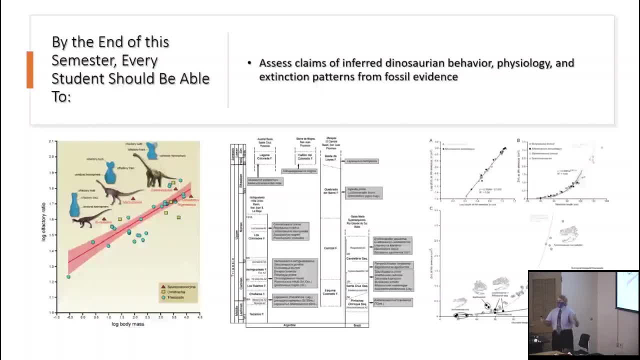 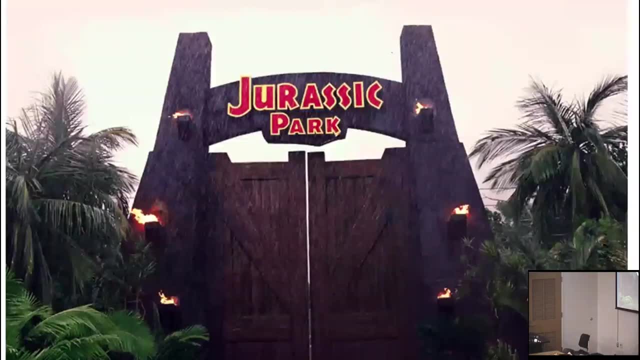 that we do in the profession to try to make sense of the bones and footprints and so forth we find. So that gives us sort of the philosophy behind the class. So let's venture into the fearsome realm of the world of dinosaurs. 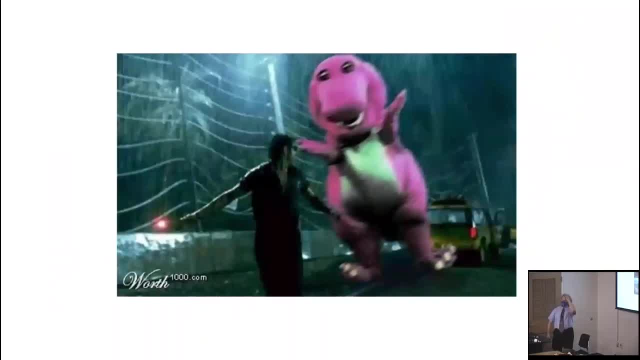 So most of the rest of this particular lecture is going to be an overview of some of the things that we'll deal with, some key concepts, and then on Wednesday we're going to start by looking at what the scientific method is. So there are ten types of people in the world. 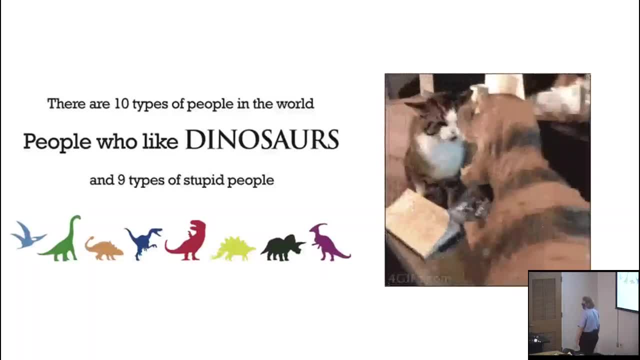 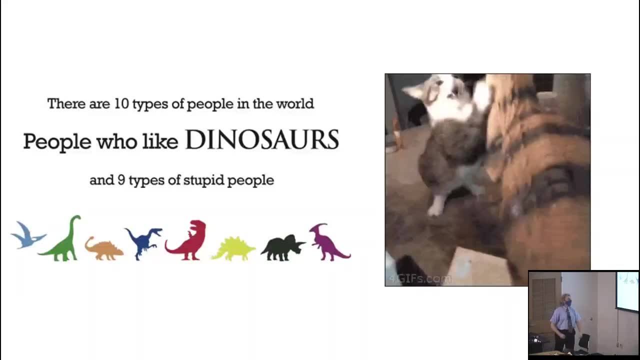 people like dinosaurs and nine types of stupid people. So don't be afraid. If you're one of these people, A congrats for taking the class and I hope to move you from one of these sorts into one of these sorts. 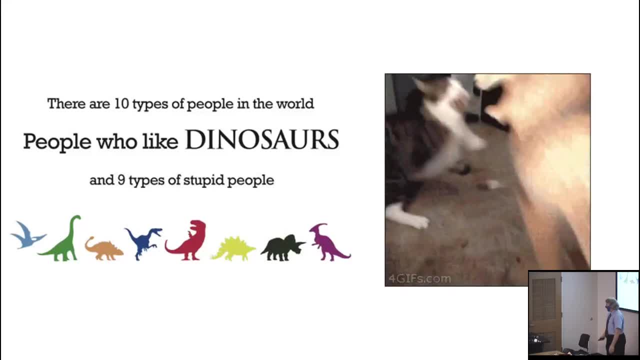 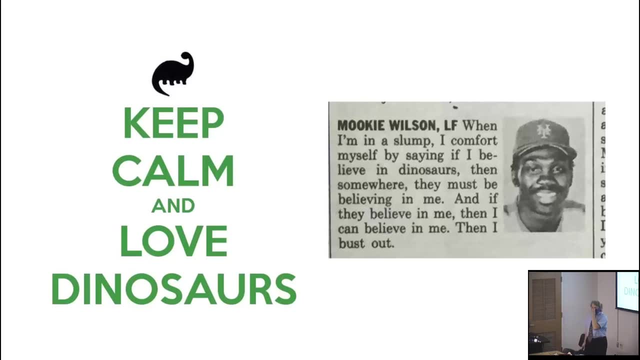 So don't be afraid The internet. dinosaurs and cats, Keep calm and love dinosaurs, and I wish this were real, but it's actually from a parody magazine. So when I get into a slump, I comfort myself by saying: if I believe in dinosaurs, 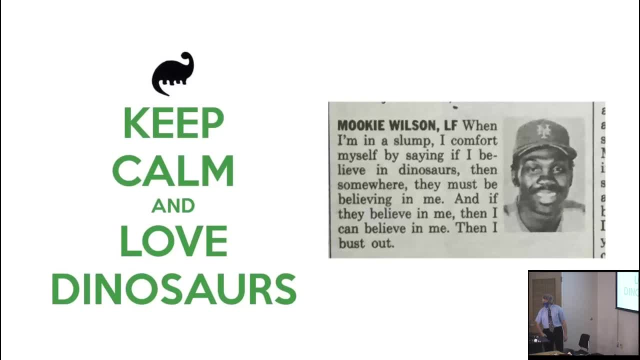 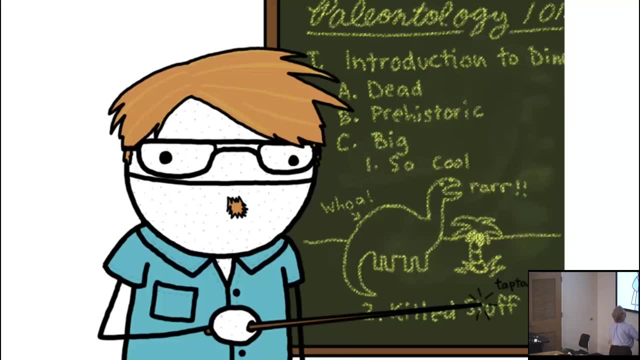 then somewhere they must be believing in me, and if they believe in me, then I can believe in me. then I bust in: Yeah, So dinosaurs dead. prehistoric big, so cool killed stuff. Well, yeah, so cool. 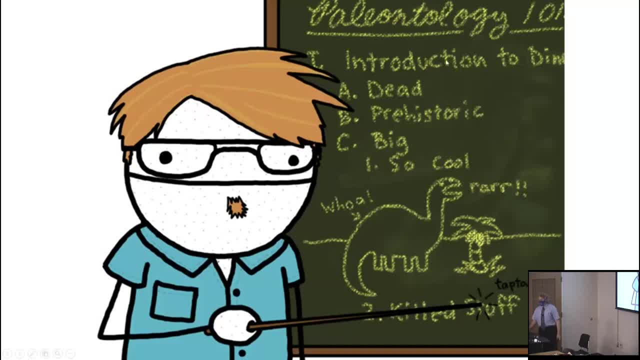 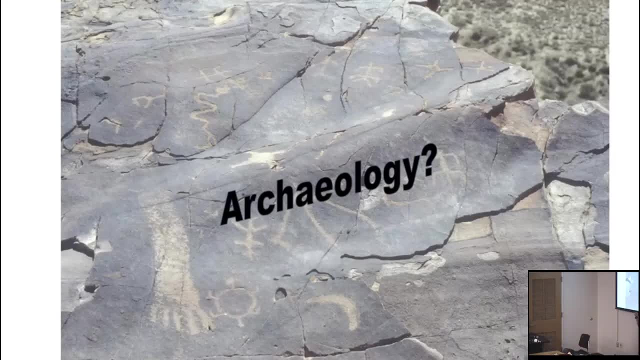 some of them killed stuff. you know, plants die. We'll see that. some of these other things, though, are not absolute. First of all, if, up until this moment in time, you said this is a course in archaeology, I would forgive you. 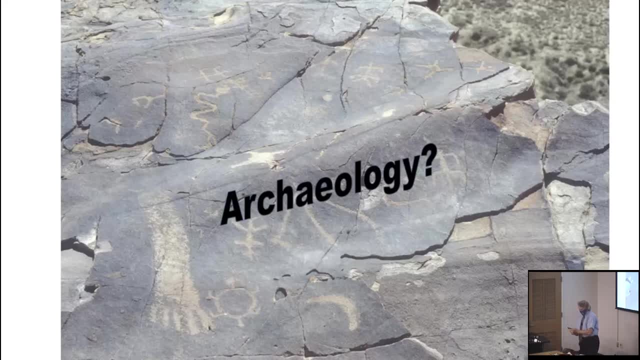 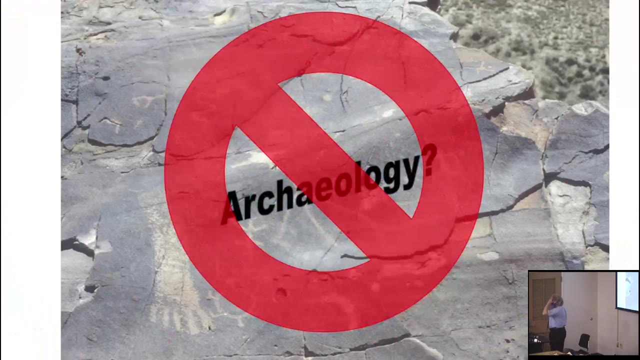 but as of 1029, I will not. This is not a course on archaeology. Archaeology is the study of ancient peoples and their artifacts, like these petroglyphs here on the sandstone, Now, the reason I was actually at that spot. 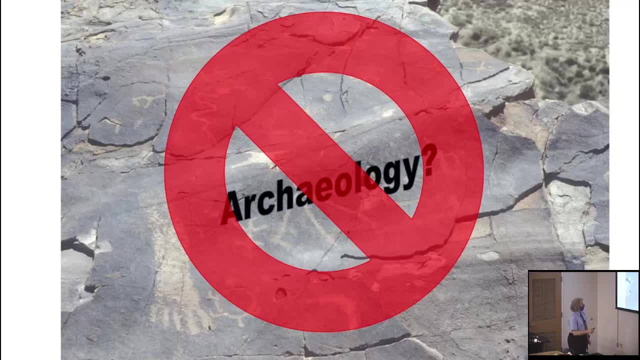 wasn't so much to look at the petroglyphs, although it was cool. by the way, What is there? Go Terps? Oh, there's a Terp. So it is not archaeology, We and archaeologists. 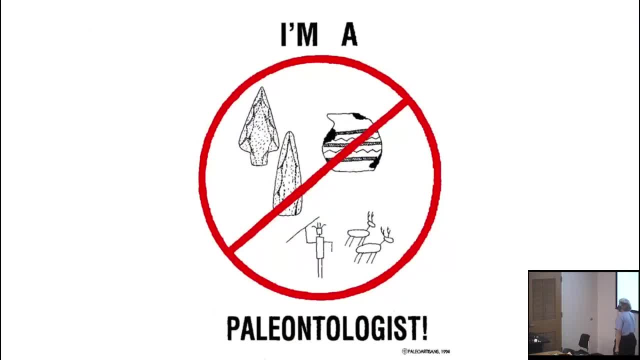 do some of the same stuff, in that we go into the field and we dig stuff up and it's old, but that's, you know, that's where it is. Archaeology is the study of ancient people and their artifacts. What we're dealing with here is paleontology. 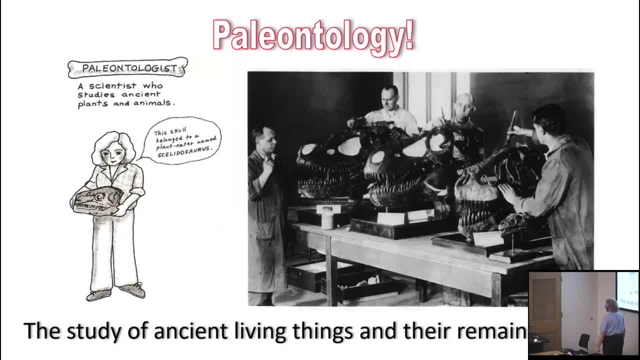 I am a paleontologist, which is the study of ancient living things and their remains or fossils, And in next week we'll go into a lot more detail as to what fossils are and how they form. I think it's next week. 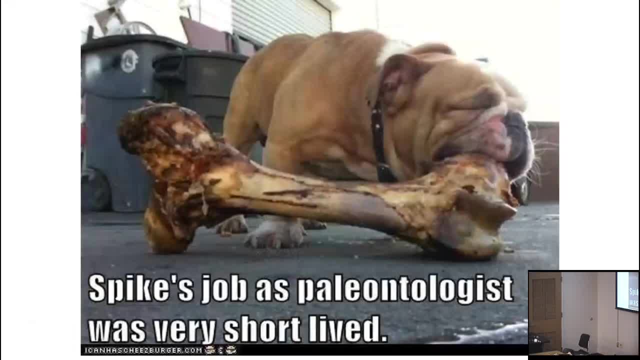 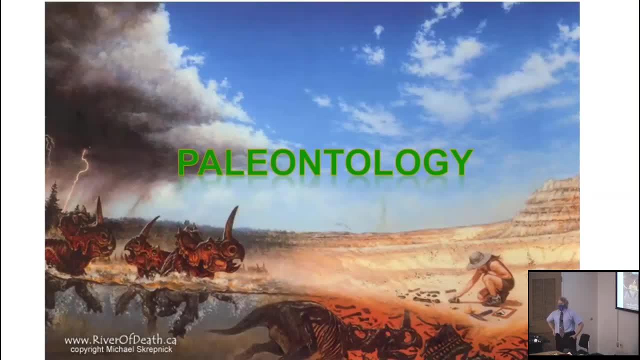 Maybe a little week after that. So yeah, Paleontology is its own science, but it's not a really big science. There aren't that many paleontologists out there, And while a natural history museum can justify having a department of paleontology, because, after all, they typically have a large number of specimens that need curation and study. a university doesn't? There are no American university departments that have that have a paleontology department. Paleontologists are either in the biology department or whatever that's called. 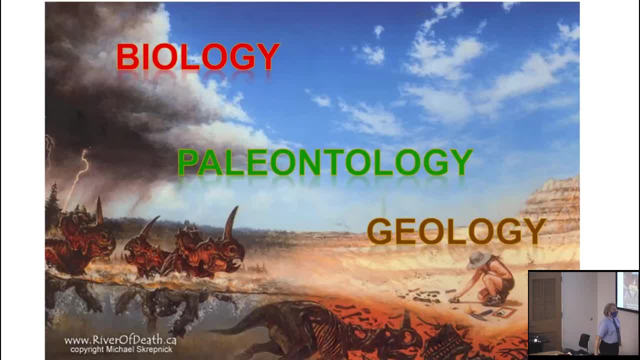 at that institution. so here, B-Sci, or in geology, or in both, because we're at the intersection, We're at the spot where we're looking at the remains of once-living things preserved in the rock record, And you need to know both. 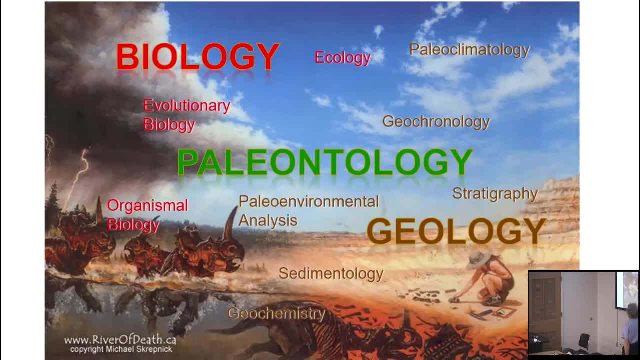 And specifically on sort of the biological end of things, we incorporate aspects of organismal biology. What's that? That's the classic disciplines like zoology and botany and so forth. Also evolutionary biology, how organisms and their lineages change through time. 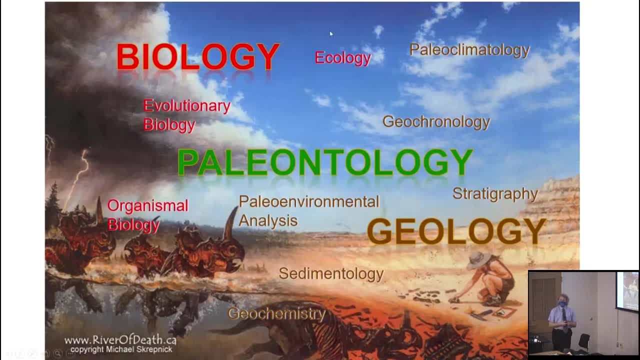 and ecology how organisms interact with each other in their non-living environment. And on the geological end of things, we deal with the fact that these are found in a particular type of rock called sedimentary rocks. We'll talk about those next week. 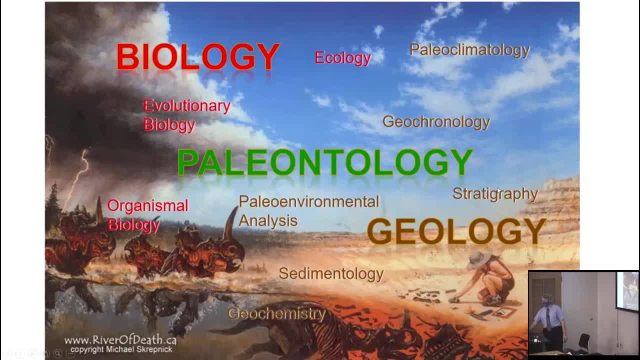 That, how those rocks are arranged, which gives us information on geologic time or geochronology, and how the data presents preserved in them, including aspects of geochemistry, help us understand ancient climates and ancient environments. So we're at the intersection. 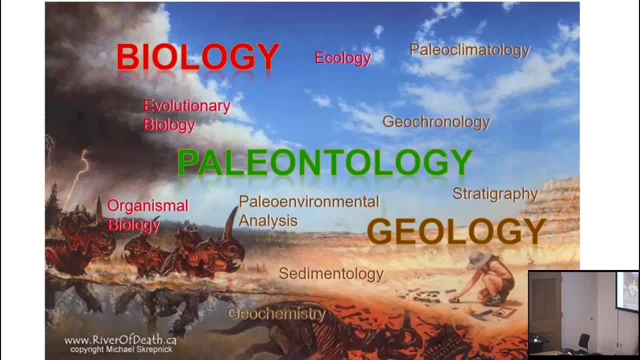 So I and my colleague John Merck are paleontologists who teach in the Department of Geology, But there is a paleontologist in the Department of Entomology here as well, Although he's retiring soon, And so that's part of B-Sci. 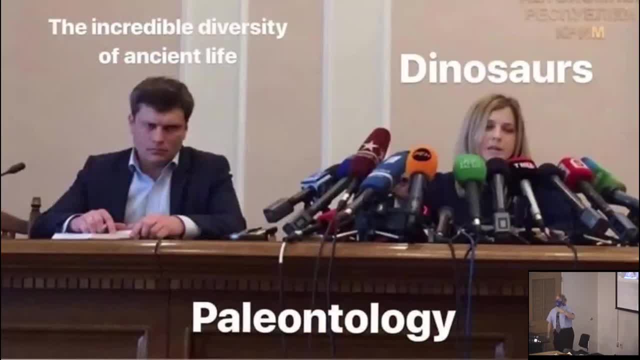 And so we're at an intersection. By the way, if any of you get really hooked, then there is a paleobiology minor that you can take, And this is actually a contributing course to that, if you want to. So the public though. 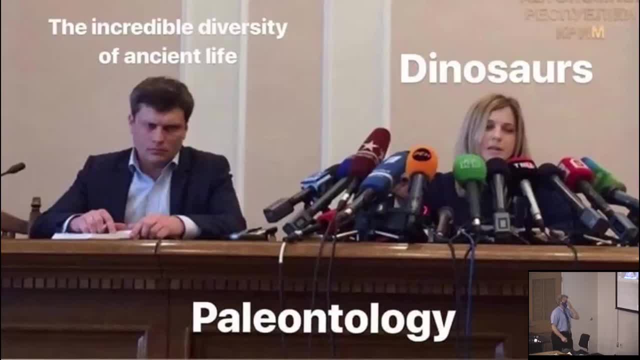 thinks that paleontology is just about dinosaurs. As a dinosaur worker, quite frankly, as a worker on the most overexposed dinosaur level, Tyrannosaurus rex, I get more attention maybe than I might otherwise if I worked on some different group. 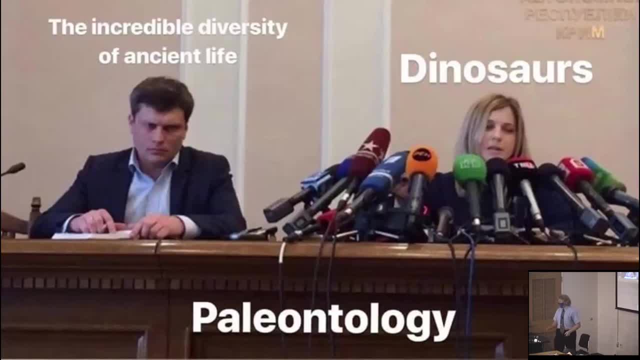 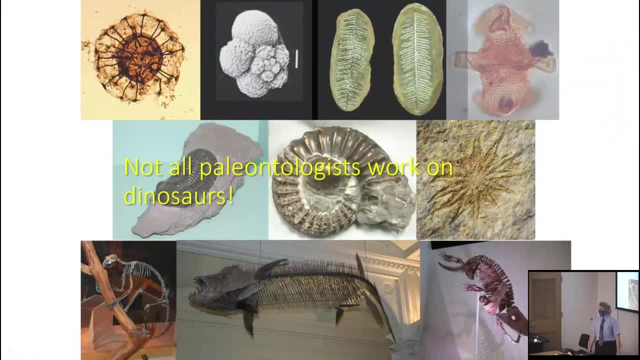 But in fact paleontology includes all the incredible diversity of ancient life. So not all paleontologists work on dinosaurs. Some of us work on pollen. I'll go through this. Oh, here we go: Pollen or microfossils. 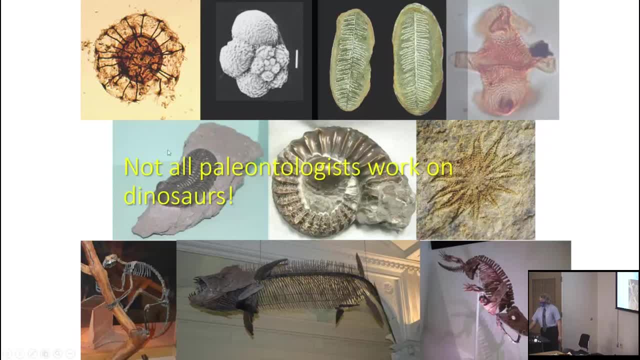 plants, invertebrates, that is, shellfish or other types of backboned animals other than dinosaurs. So things like you know: fish, amphibians, mammals or even non-dinosaurian reptiles. So none of the creatures. 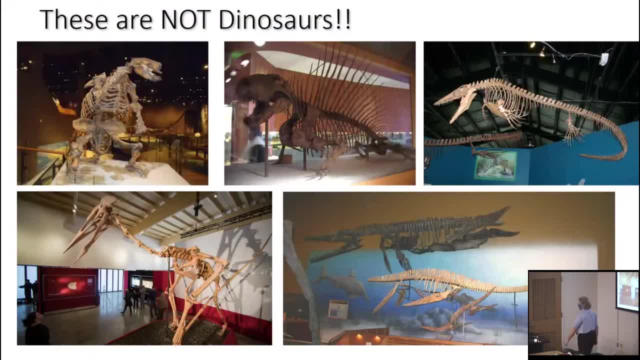 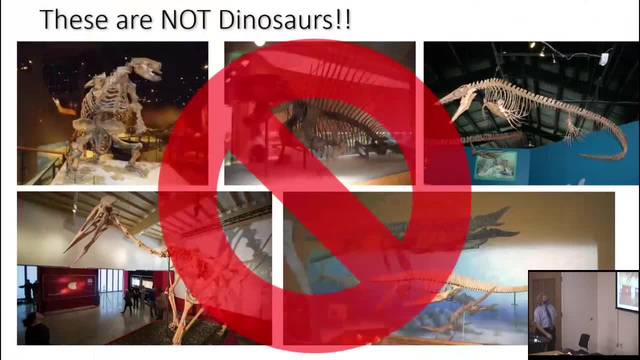 on this slide are dinosaurs, although if you go to a museum you will overhear people say, look at those cool dinosaurs, But they're not. So the giant ground sloth is a mammal, The thin back here, Dimetrodon. 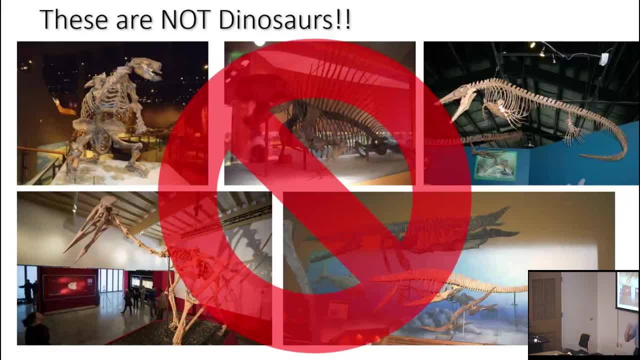 is not even a reptile, It is a proto-mammal. It's on our lineage, closer to us and kangaroos and duck-gilled platypus and whales than it is to a lizard, a snake, a turtle. 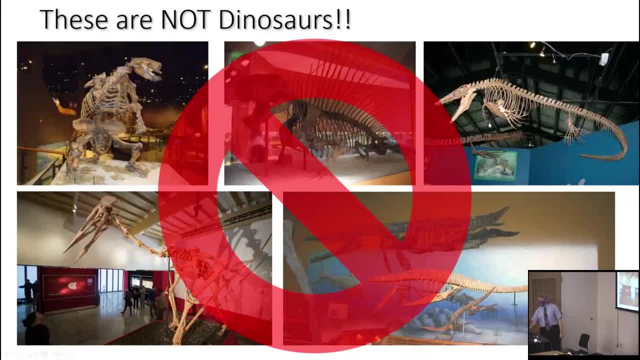 a crocodile, a dinosaur, The Mosasaur here, that's an honest-to-goodness lizard And it's a member of the lizard group. These marine reptiles are their own branch of extinct reptiles, coincided in time with the dinosaurs. 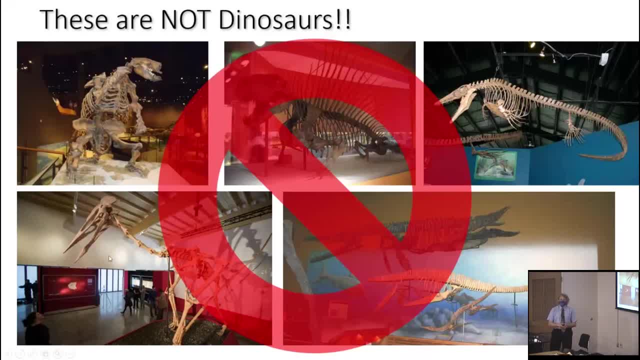 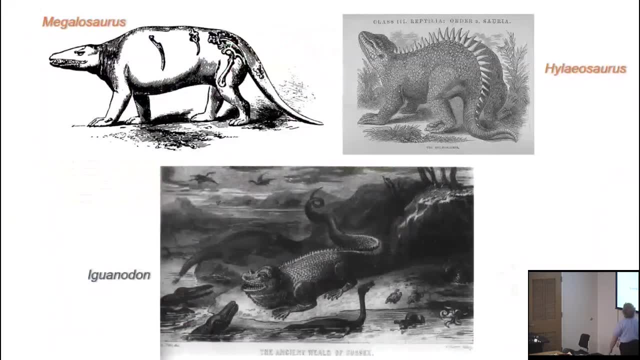 but not dinosaurs. And the pterodactyls and the other pterosaurs- not dinosaurs, but really, really, really, really, really, really close relatives. So what is a dinosaur, As we'll talk about at the end of this week? 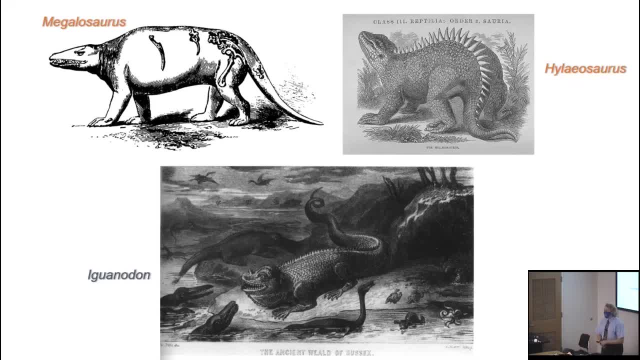 the concept of dinosauria began in reference to these three types, these three genera, as they're called, in the early 19th century, Three different reptiles discovered in rocks of the Jurassic- the Jurassic and Cretaceous of southern England. 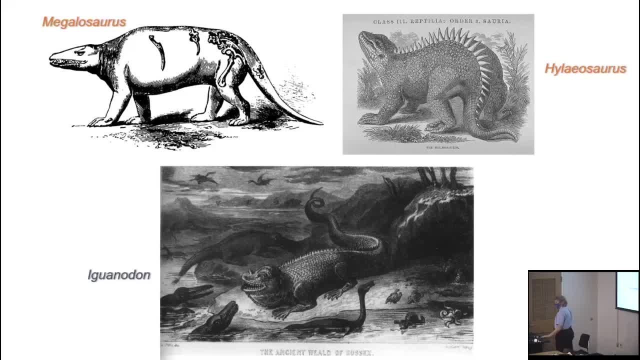 specifically Megalosaurus, Iguanodon and Hylaeosaurus. Now the three of them don't look, didn't look anything like these illustrations you see here. These are very early illustrations. I'll talk about the history. 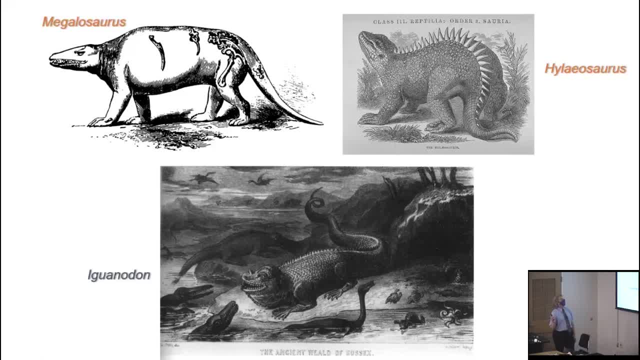 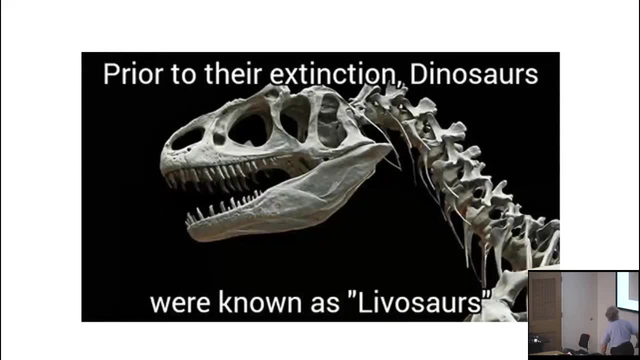 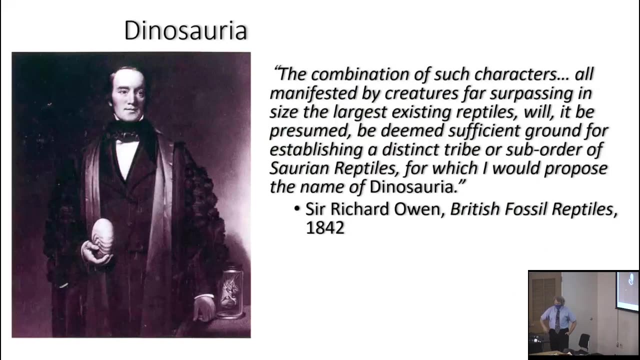 of their discovery on Friday And they were used to coin the name dinosaurs. so no, Prior to their extinctions they were not known as liposaurs. So dinosaurs, The word dinosauria, the name dinosauria, is not some ancient word. 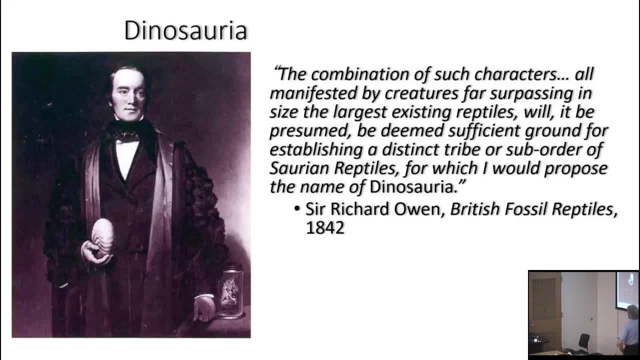 You know, Caesar wouldn't have heard of it, Leonardo da Vinci would never have heard of it, Thomas Jefferson would have never heard of it, although he would have been really interested And he almost lived late enough in time to hear about it. 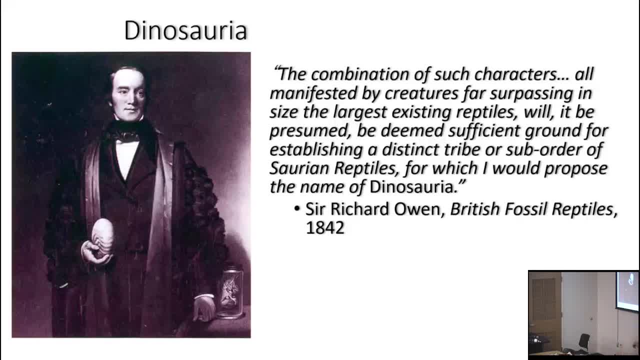 And this is the paragraph in which that word is coined. So I'm not going to do a British accent here, but I'm going to start with Richard Owen. He's the guy who named dinosauria And he says the combination of such characters. 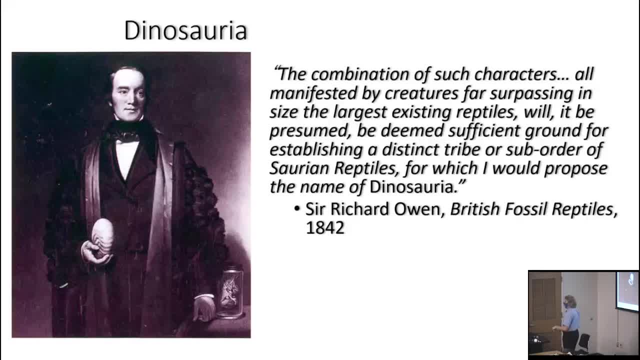 in this case, character means traits or characteristics all manifested by creatures far surpassing in size the largest existing reptiles, will be presumed the deemed sufficient ground for establishing a distinct tribe or suborder of saurian reptiles, lizards and crocodiles. 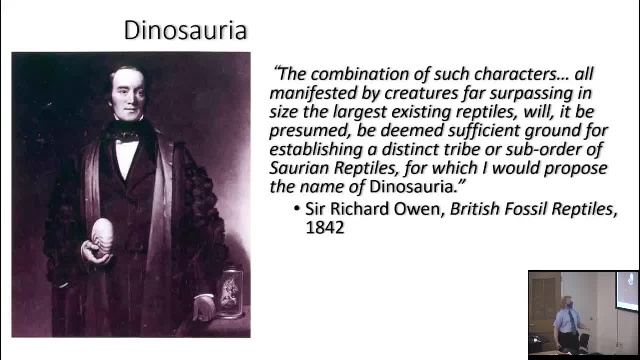 and so forth, for which I would propose the name of dinosauria. And you go down to the little footnote associated with that and it's from two Greek words, Dinos, which is fearfully great. Sometimes you see it translated as terrible. 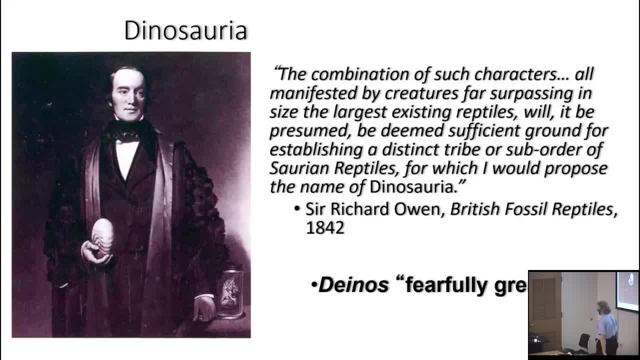 but if you actually go to the paper, he says fearfully great, which is not merely big, great, but fearfully great. So Victorian speech were scary big And sauros lizards. so the fearfully great lizards- We'll come back to that. 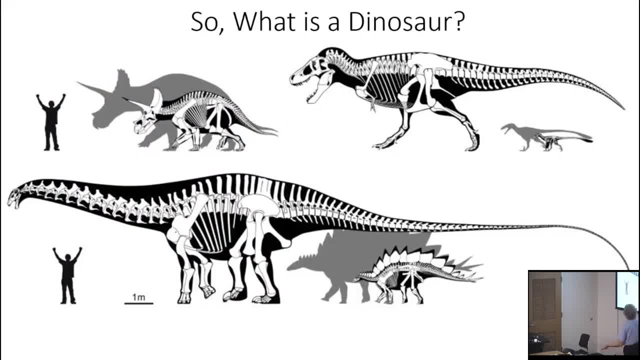 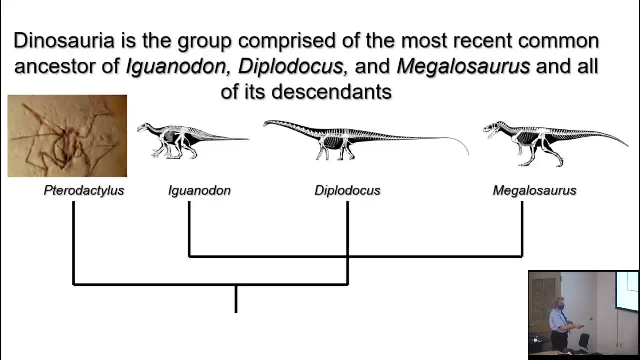 So that's the etymology of dinosauria, the guy who named it. but what is a dinosaur? Well, here's the technical definition right now. I'm sorry that Scott Hartman's name got trailed off here. I'm trying to make certain. 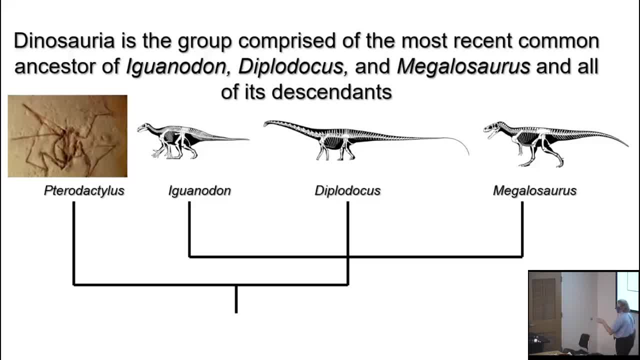 that I give you the attribution for the artists of the skeletons and the life reconstructions. So dinosauria is the group comprised of the most recent common ancestor of Iguanodon, Diplodocus and Neglosaurus and all of its descendants. 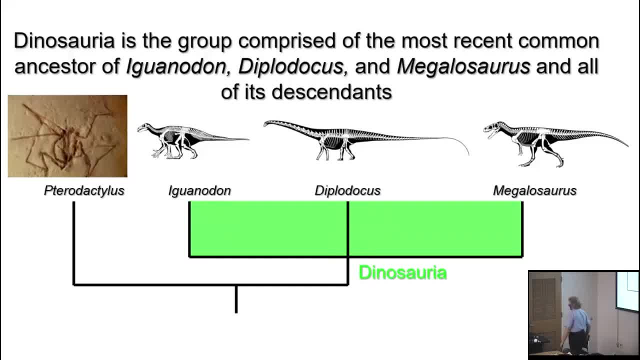 So on a family tree like this, if you descended from the common ancestor of these three, from this branch point that connects these three, you're a dinosaur. If your lineage branched off before that common ancestor split from each other, then you're not a dinosaur. 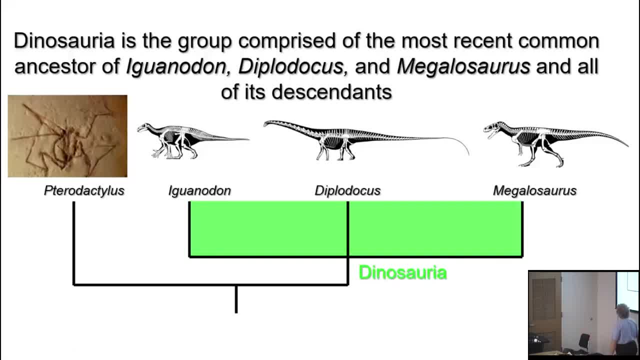 So pterodactyls, like pterodactylus here, are not dinosaurs, Not because they're small, not because they flew, but because they are not the descendants of the most recent common ancestor of Iguanodon. 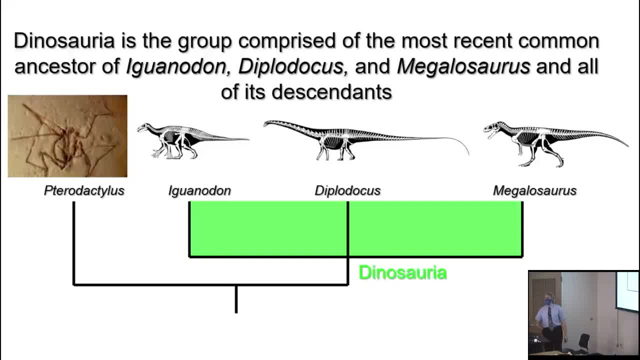 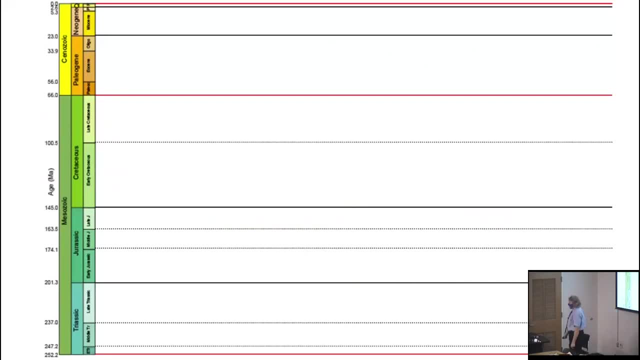 Diplodocus and Neglosaurus or one of its descendants, in this context. So that's what a dinosaur is. We'll come back later on to why this definition is chosen and what that means. So let's take a look here at the geologic time scale. 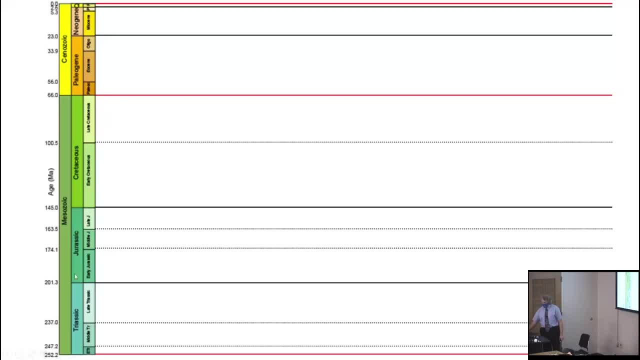 So the beginning of what's called the Mesozoic era, the age of reptiles, is right down here, Immediately after one of the greatest extinctions in the history of life. we are at the top. The oldest known dinosaurs are from around. 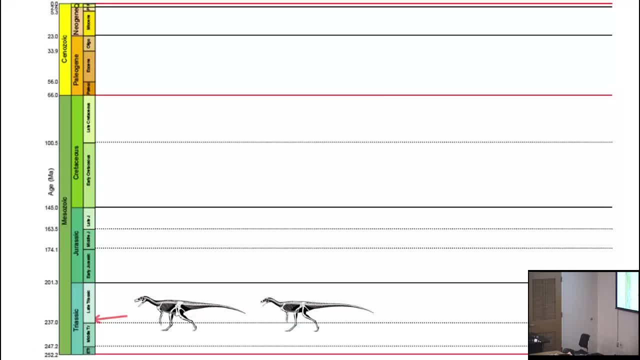 about 235 million years ago, sort of right around the time of an epoch, as it's called, a unit of time called the Middle Triassic ended and the Late Triassic began, known as the Mesozoic Era. It's known best. from South America. The classic dinosaurs of the Jurassic are from about 150 million years ago, known especially from places in western North America. So this would include Stegosaurus, Diplodocus and Allosaurus, and Apatosaurus and its cousin. 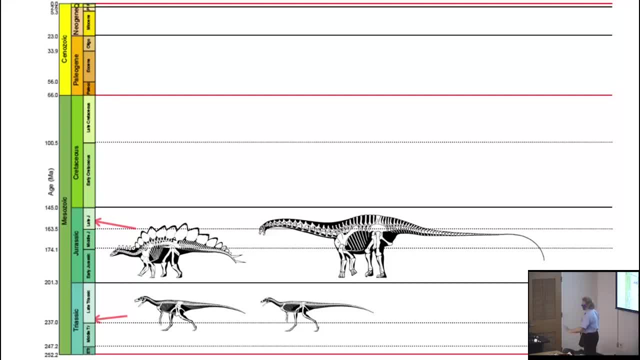 Brontosaurus, which is a legit dinosaur again. We'll talk about that later on. The last of the giant dinosaurs, things like Tyrannosaurus, Triceratops and Montasaurus are from about 66 million years ago. 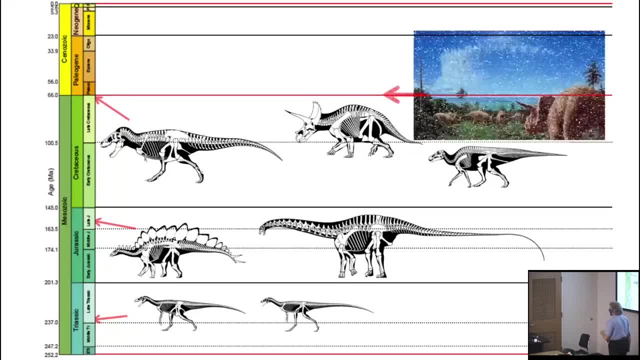 and individuals of those species would have if they were facing the wrong direction, or right direction from your point of view- witnessed the Great Catastrophe at 66 million years ago, And we are here, And so, as I've been saying since the 90s, 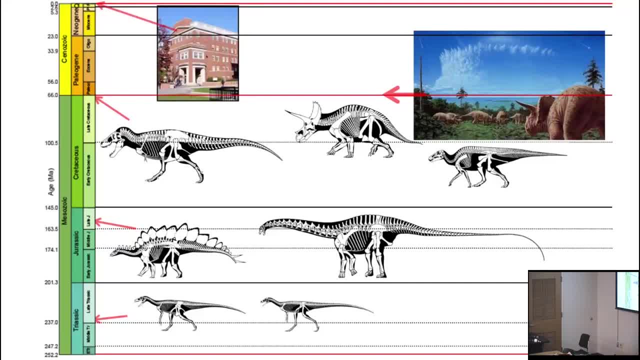 Tyrannosaurus rex is closer in time to us than it was to Stegosaurus by about 15 million years And Stegosaurus is the largest dinosaur in the world. It's the largest dinosaur in the world And Stegosaurus is only. 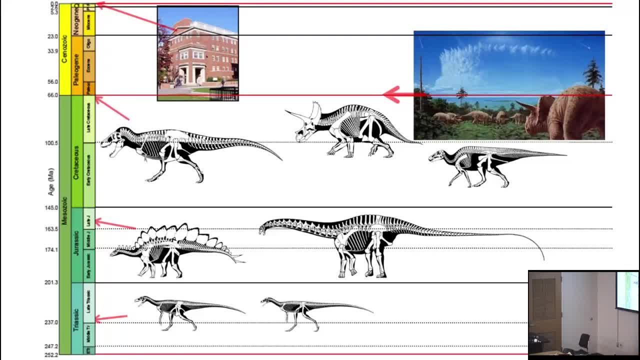 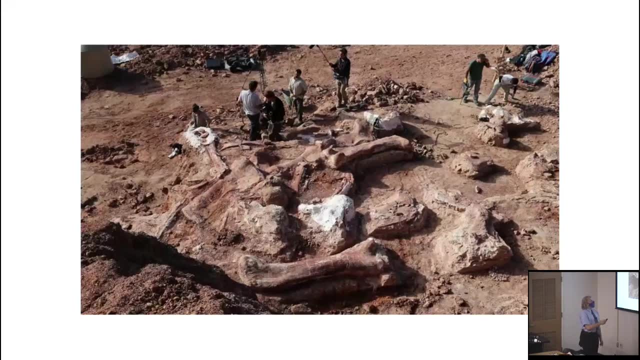 halfway back from Tyrannosaurus to the beginning of the age of dinosaurs, So really it's better to think of the ages of dinosaurs. Of course, what we mostly know about dinosaurs are their bones. So of course, famously, some dinosaurs. 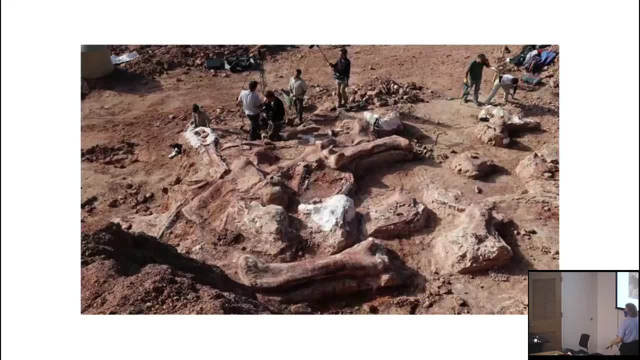 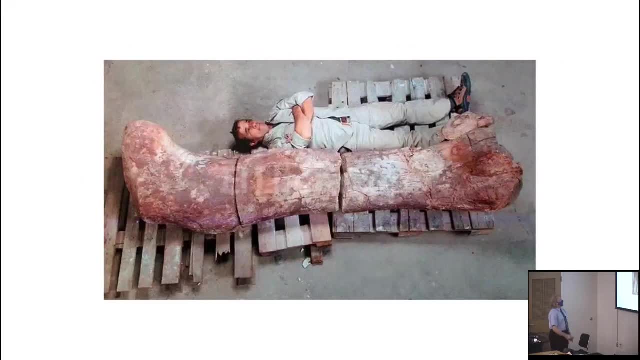 are tremendously huge. Indeed, that was one of the attributes that Owen first recognized: that they were far surpassing in size the largest animals in the world. So this is this phenomenon, that if you ever have the femur, that is, the thighbone. 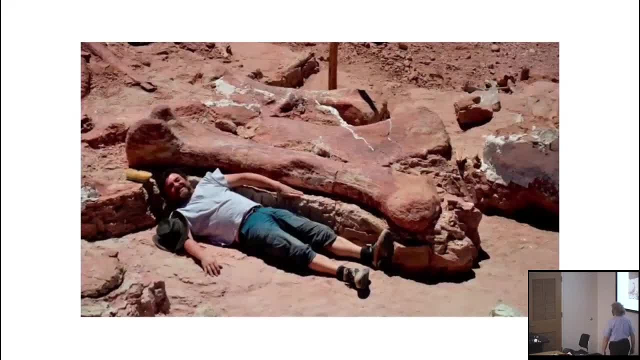 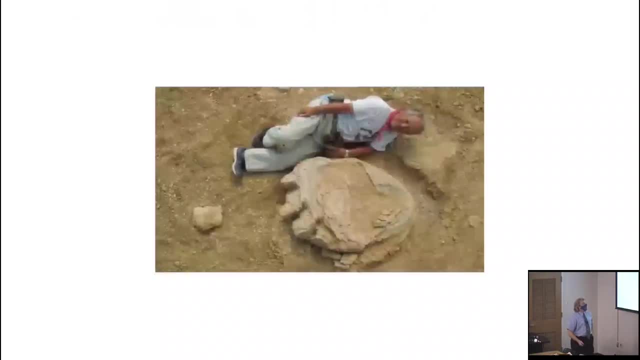 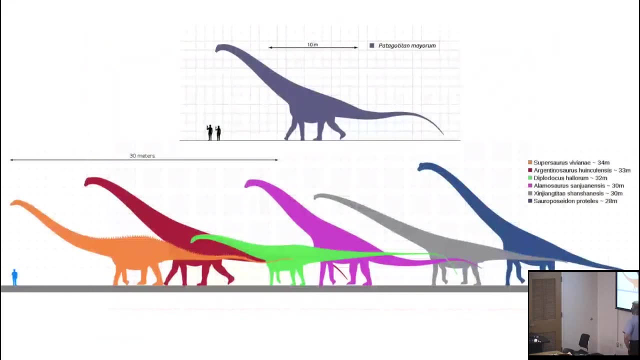 of a large dinosaur, you are required to lie next to it in its scale arm. See, Okay, So gigantic animals, larger than the largest land-living animals today, And we also have gigantic footprints that show us these huge creatures who are out there. 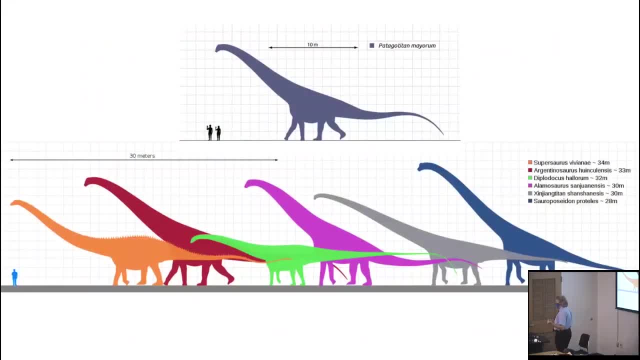 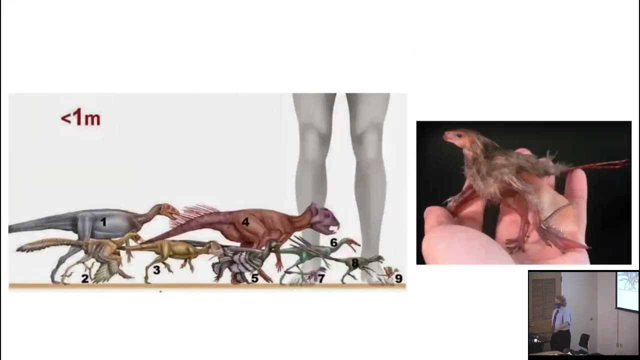 And of course that's really impressive. And the mass of maybe not the largest living species of whales, but more massive than a herd of elephants, that's truly tremendous. But not all dinosaurs were huge. Many of them could stand at the palm. 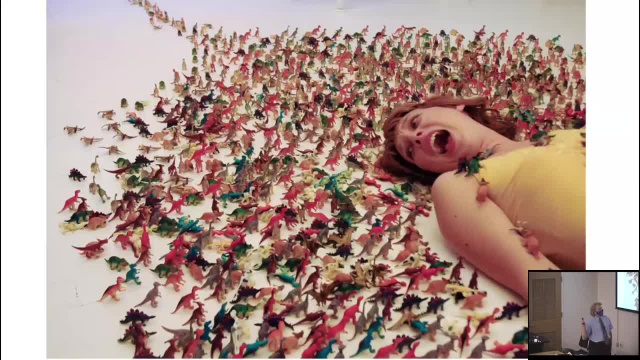 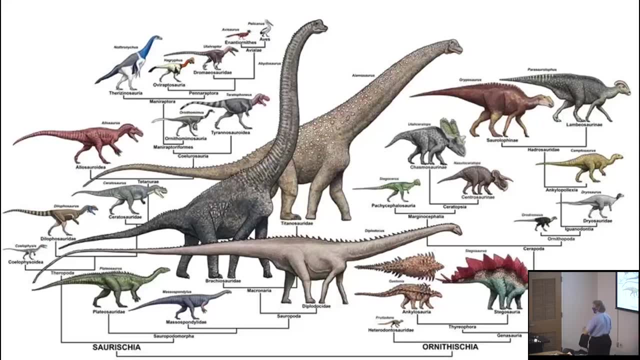 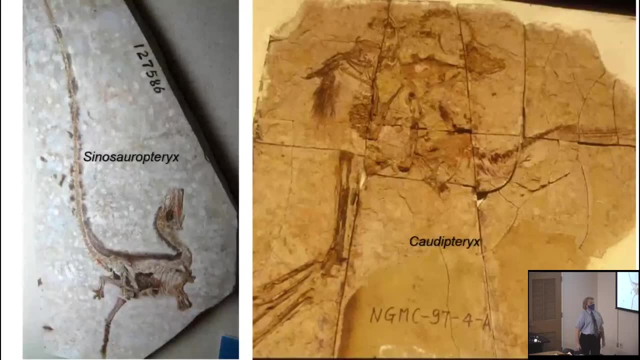 of your hand, So don't be afraid of the little dinosaurs either. In fact, it's an extremely diverse group. Even with that specific definition of those three branches, there's an amazing amount of diversity of animals within them, And indeed, 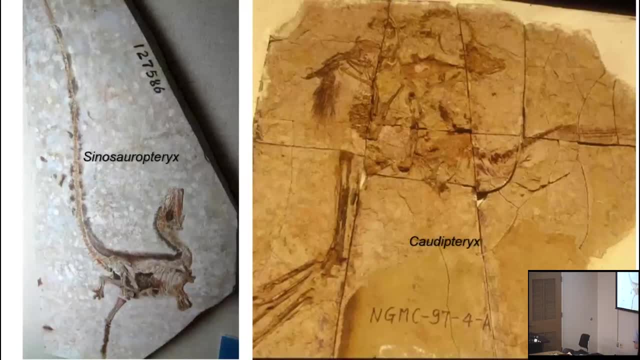 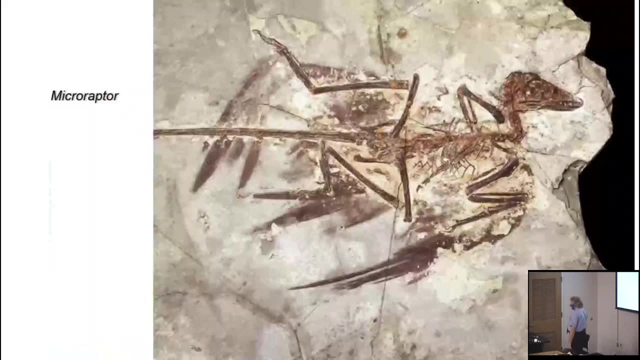 some of the small ones we now know are covered by either fuzz or honest-to-goodness feathers. Indeed, some of those are as feathered as, and possibly even flying like, modern birds, And indeed this is a far more likely. 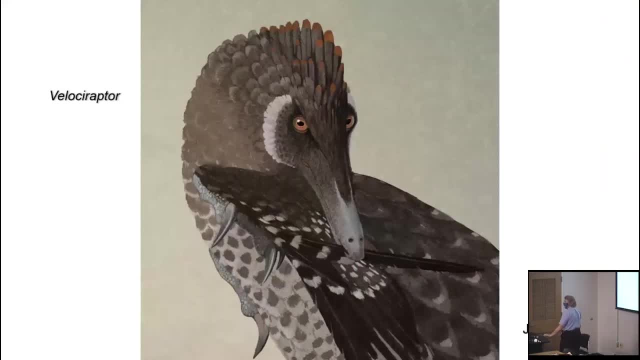 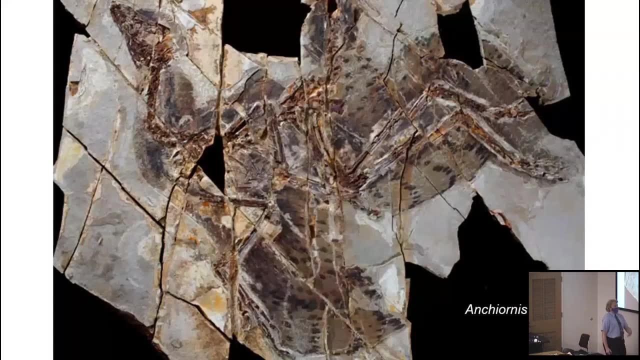 restoration of Velociraptor a feathered dinosaur than what you see in the original movies. And when you get to one point in the family tree it becomes extremely difficult to say: are you dealing with a non-bird dinosaur or a? 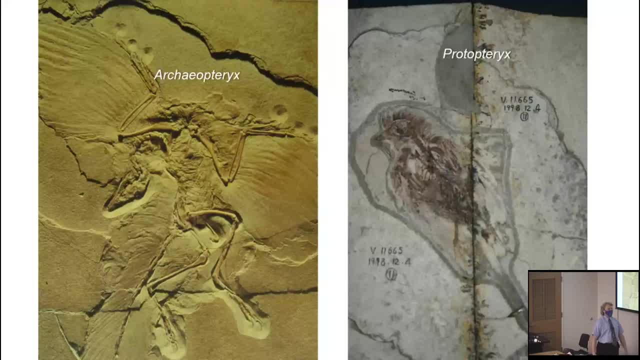 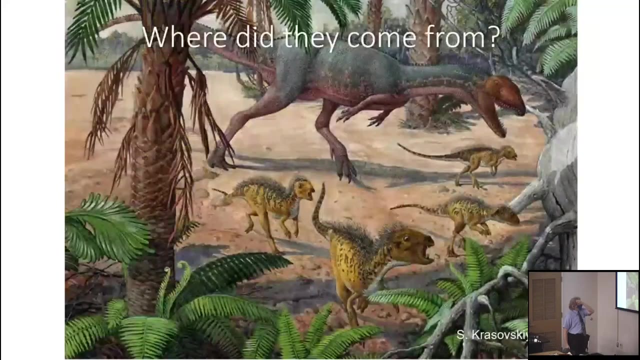 true bird And indeed, as we'll see, don't think of birds as different from dinosaurs. They are part of this dinosaurian family tree And indeed they split between birds and other dinosaurs to the origin of fully modern birds. So 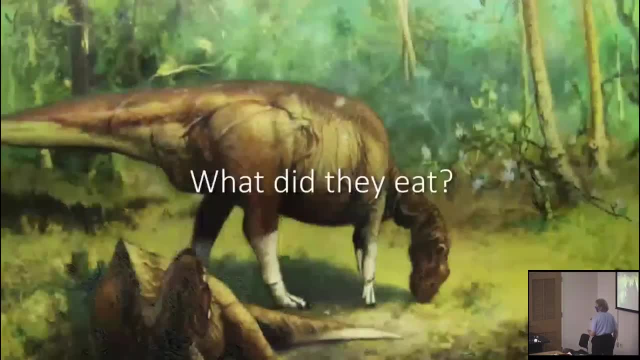 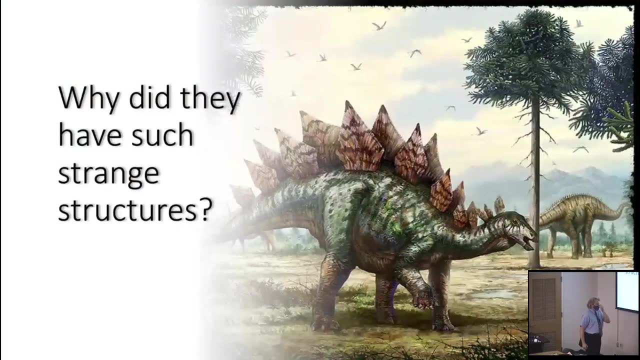 some of the main things, to wrap this up, that we'll talk about. Where did dinosaurs come from? What were their ancestors? Where did they fit in the family tree of life? What did their evolutionary and ecological reasons for? looks really awesome. 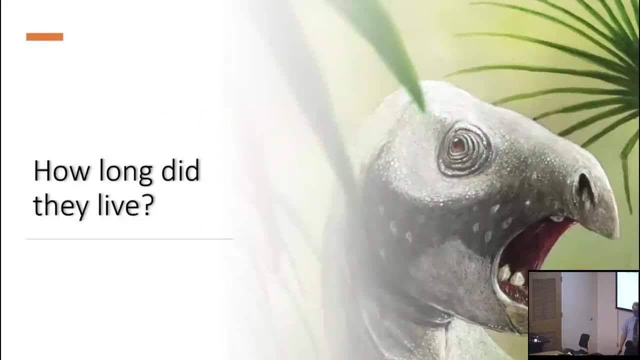 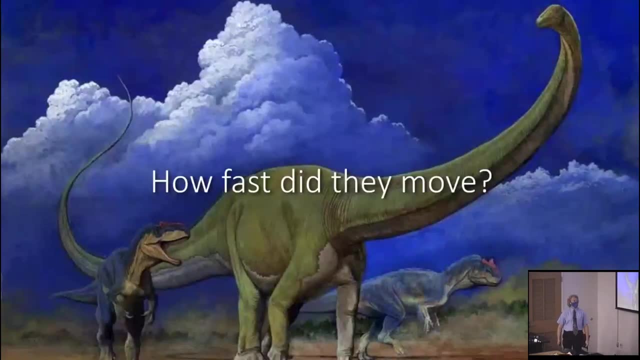 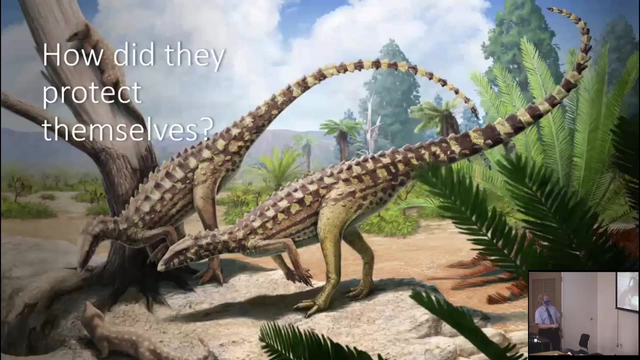 How long did an individual live? You know, how long did a Tyrannosaurus or a Stegosaurus or whatever live? How fast did they move? As you might imagine, different species have different answers for that. How did they protect themselves? 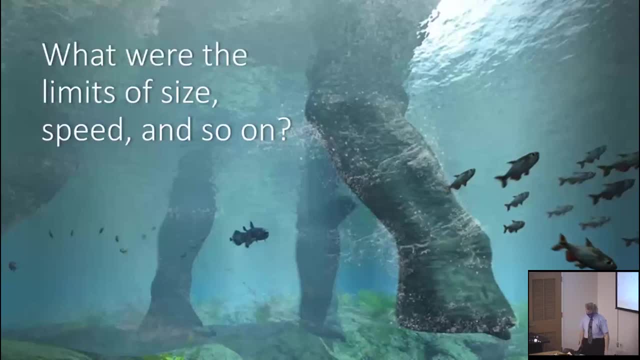 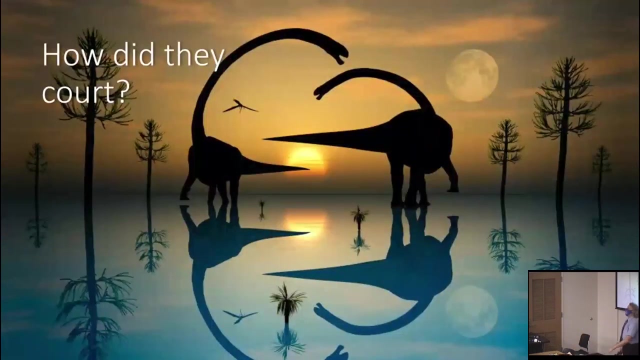 That's one of the cool aspects of dinosaurs is that the larger ones tend to push the physiological limits of a land animal, In this case one that's walking a little bit through the water. but it's a land animal, How did they court? 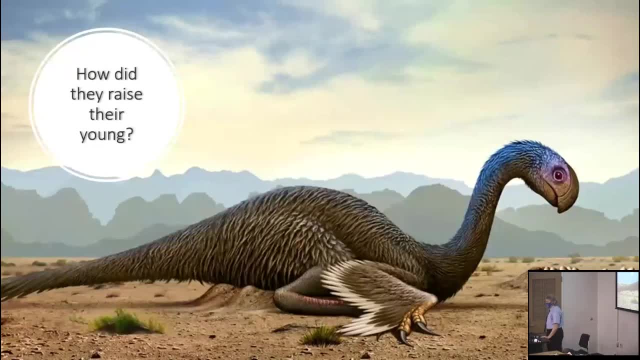 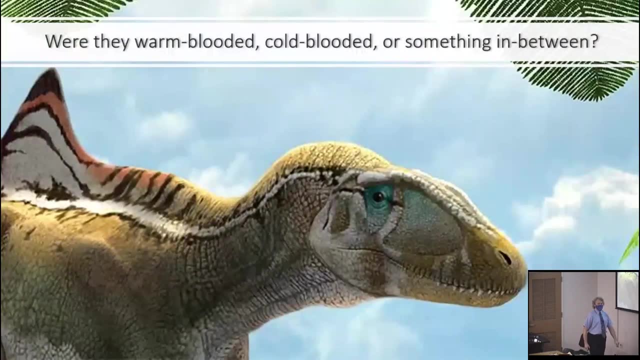 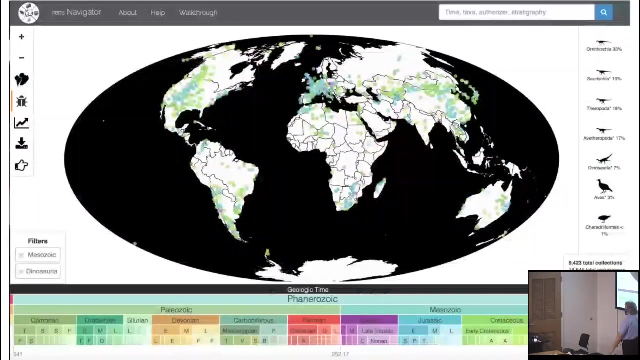 and how can we tell? If you have individuals that don't live in a land animal, you can't tell them what's involved with them. Were they warm-blooded, like mammals, or the living part of the dinosaurs, the birds? Were they cold-blooded? 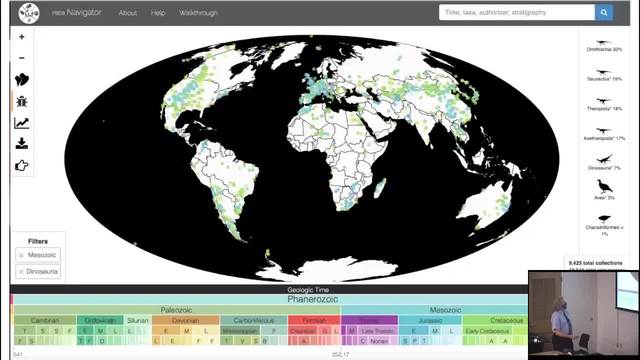 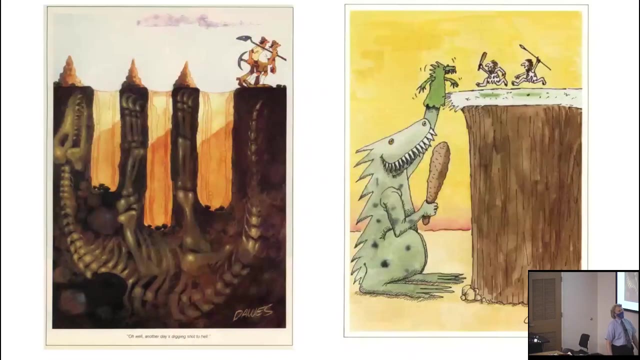 like lizards and snakes and turtles, Or were they something in between? And, ultimately, what happened to them? So these are some of the questions that we need to ask ourselves in order to find the answer to this question. The answer to this question. 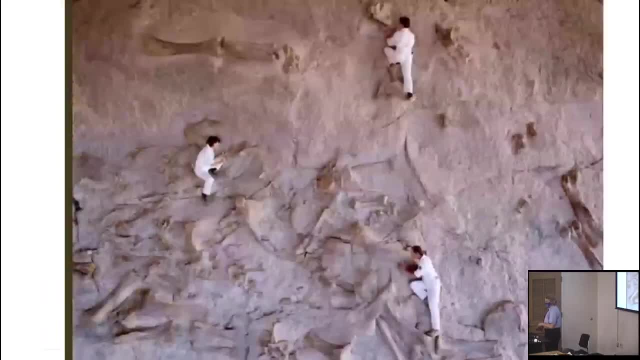 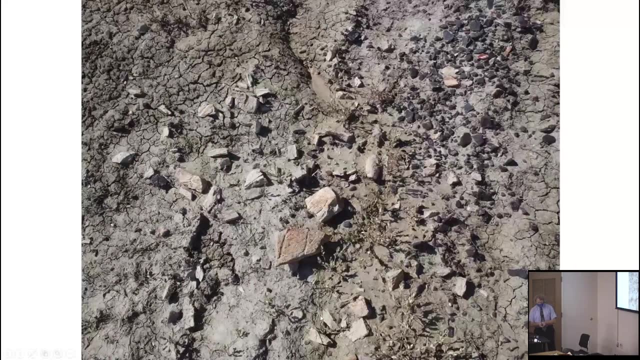 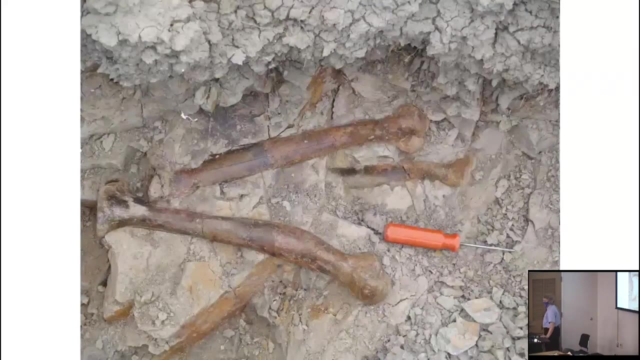 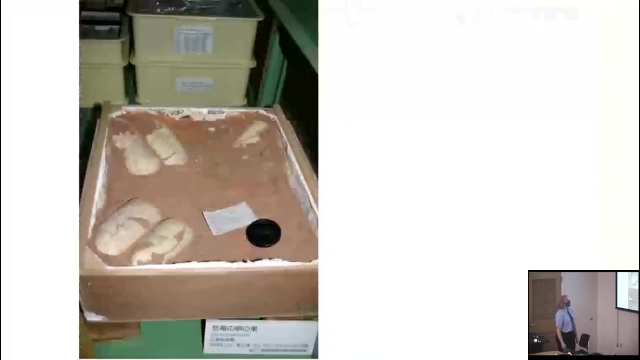 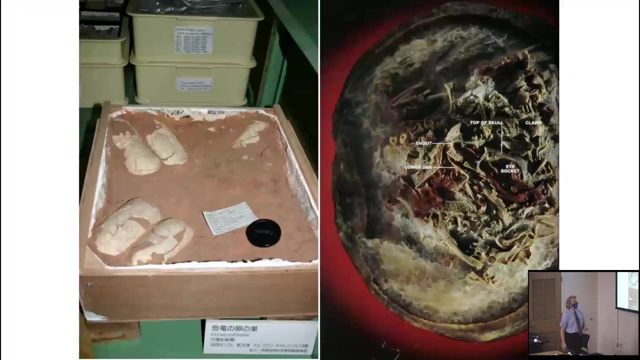 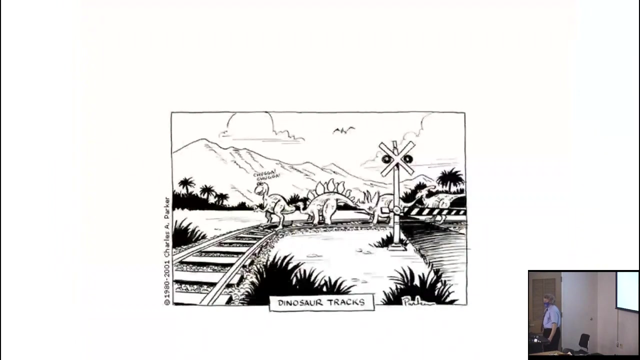 is that we have to find the answer to this question. So we have to ask ourselves what is the answer to the question that we had to come up with, And what we have to find is that we can find the answer to this question in one. 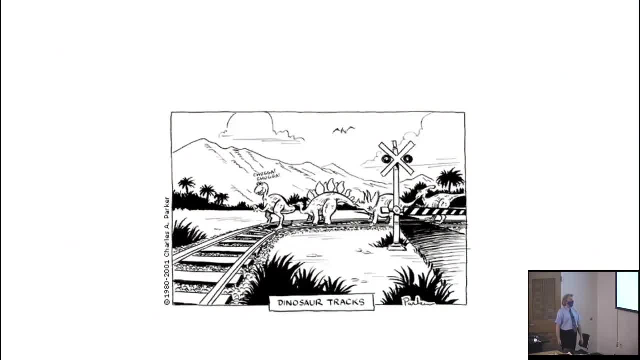 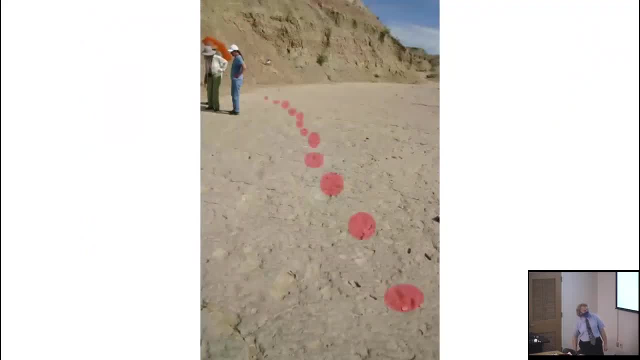 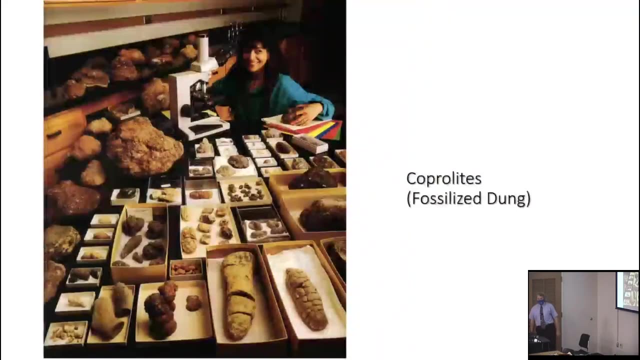 studies are their tracks, the traces they left behind on the ground, for instance, like footprints. Here's an allosaurus track. Here's a trail and a highlight in red of dinosaur tracks, when it was walking on a beach in what's now Wyoming, And even what they. 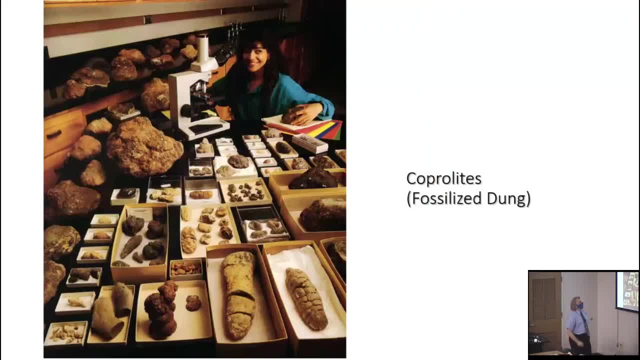 really left behind, which is poop, fossilized dung, coprolites- literally crap stones. This is Dr Karen Shin, one of my colleagues. She is the world authority on dinosaur crap And, honest to goodness, that's a good thing to study.